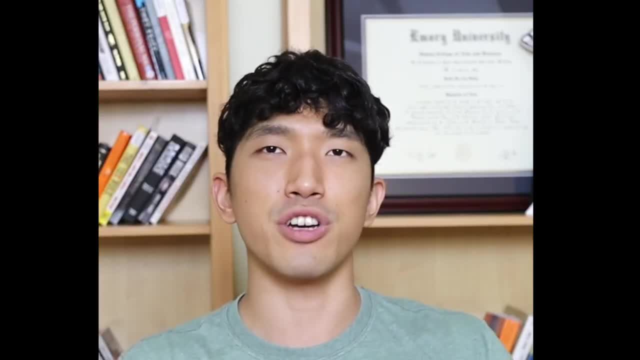 going to be a word problem. And to solve all these word problems, all you have to do is just convert words into numbers. That's it. If you can convert words into numbers, you are going to be able to solve these word problems. So let's go over this fail proof method. 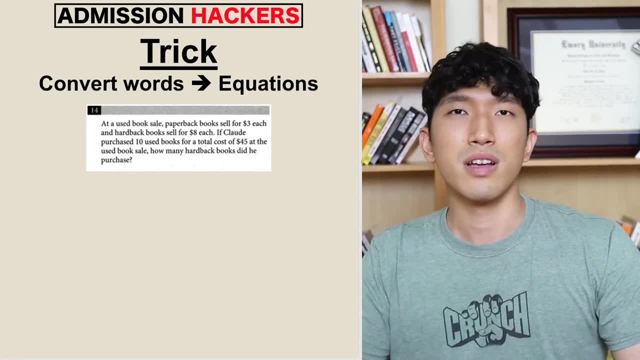 and solve these word problems. And to solve all these word problems, all you have to do is just convert words into numbers. If you can convert words into numbers, you are going to be the king of word problems. Nothing's going to be impossible. So let me show you what I exactly mean by. 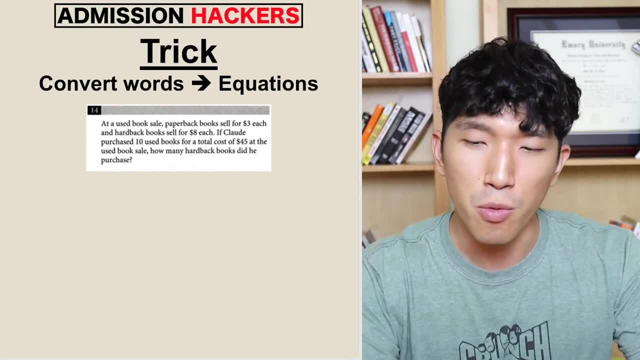 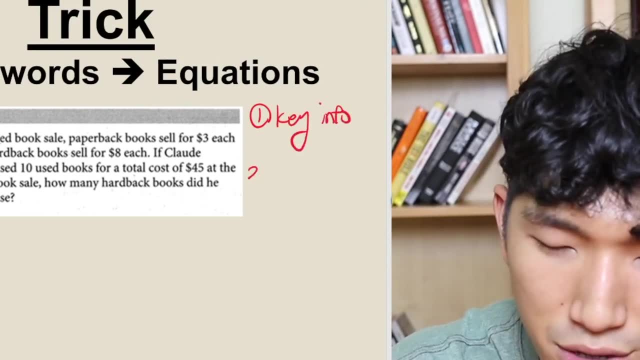 converting words into numbers. Let's dive into this question. So, whenever it comes to word problem, the first thing you want to do is going to be identifying key information. Okay, And based on the key information, what we're going to do is we're going to create equations. Okay, So let's. 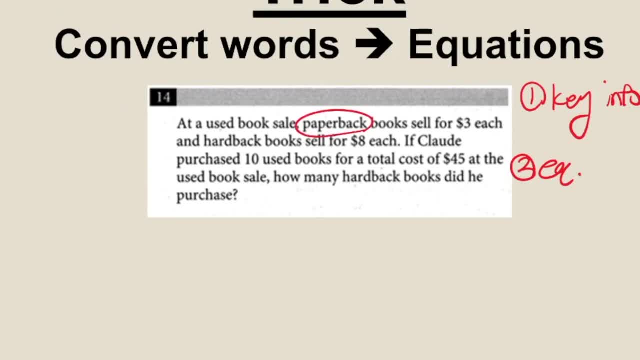 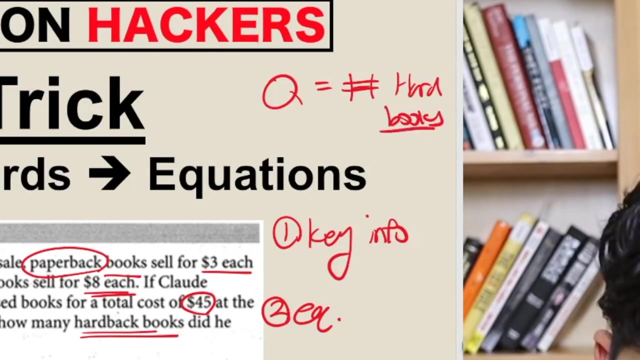 look at this question for an example. At a used book sale, a paper book sells for $3 each and a total cost of $45.. At a used book sale, how many hard books did he purchase? So what we are looking for in this case is the number of hard books, hard books, right. So the first thing we have to do is 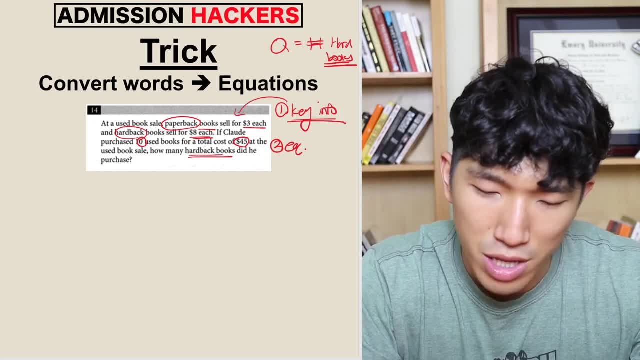 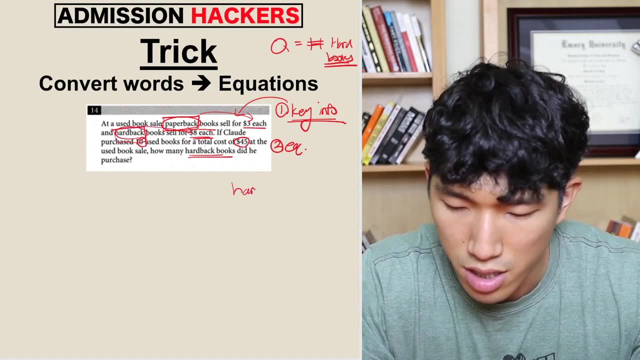 identify key information, And we did exactly that. Okay, So we know that paperback is going to be $3 each and hard books is going to be $8 each, So we're just going to write that down: Hard is going to be $8 each. 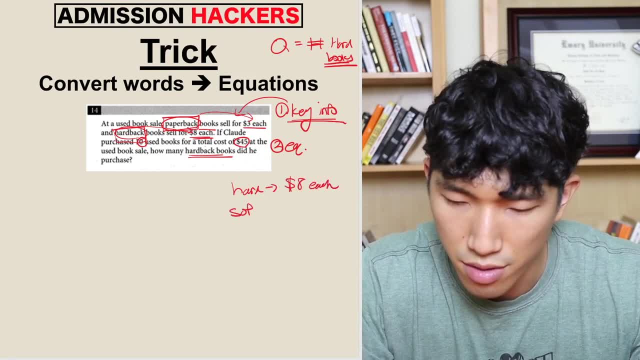 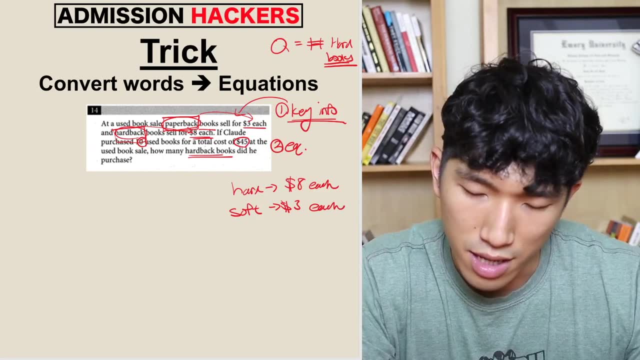 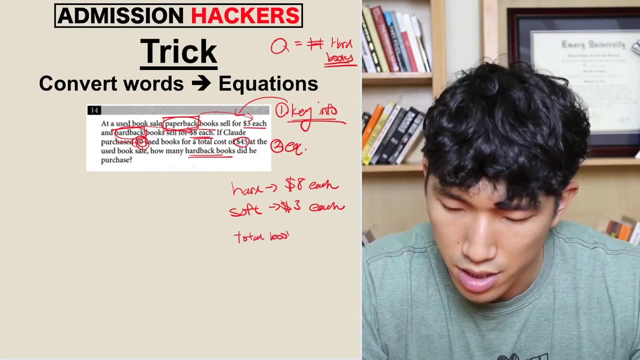 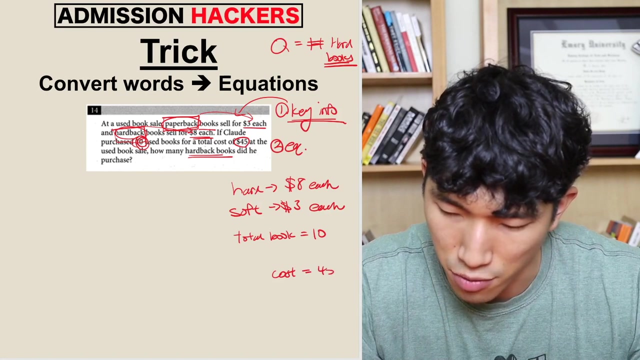 And soft is going to be $3 each, Okay, And another thing that the question tell us is that the person purchased 10 books total, So we know that total book is going to be 10, right, And the total cost is going to be $45, right. And based on this key information, what we're going to do is we're going 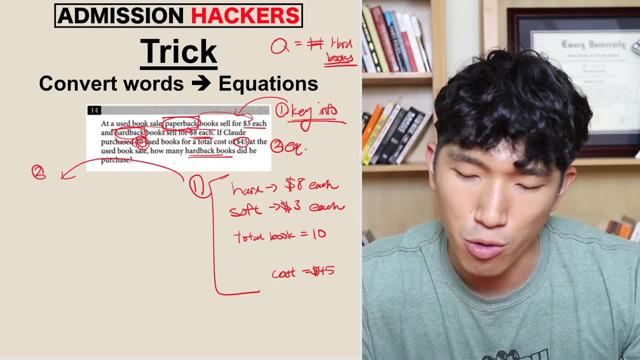 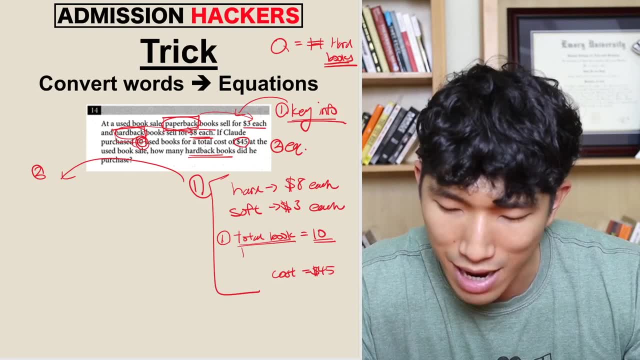 to create an equation. So let's look at this question for an example At a used book sale equations. okay, So our first equation is going to be based on the total number of books, and the total number of books is going to be 10.. And we know that total number of books is made out of 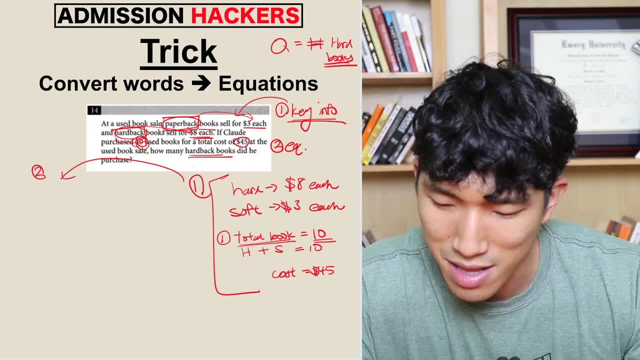 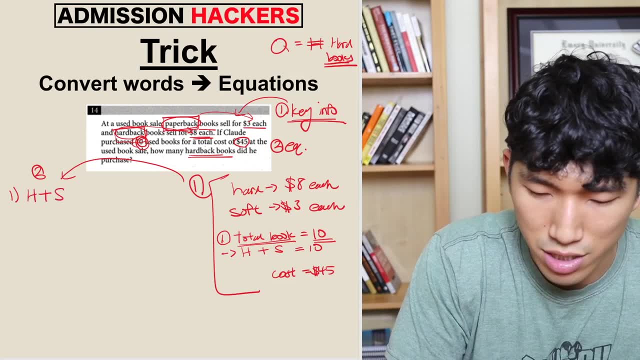 hard books plus soft books, right? And that's going to equal 10.. And that's going to be your first equation, right there, right? So our equation number one is going to be H plus S, which is number of hard books plus number of soft books, And that's going to equal 10.. And the second: 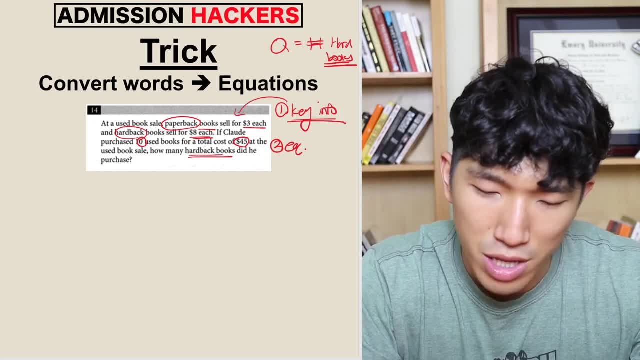 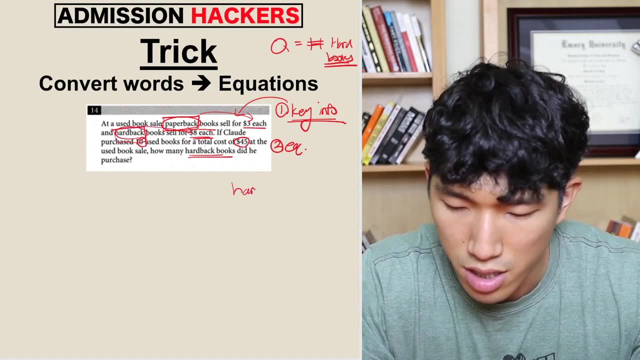 identify key information, And we did exactly that. Okay, So we know that paperback is going to be $3 each and hard books is going to be $8 each, So we're just going to write that down: Hard is going to be $8 each. 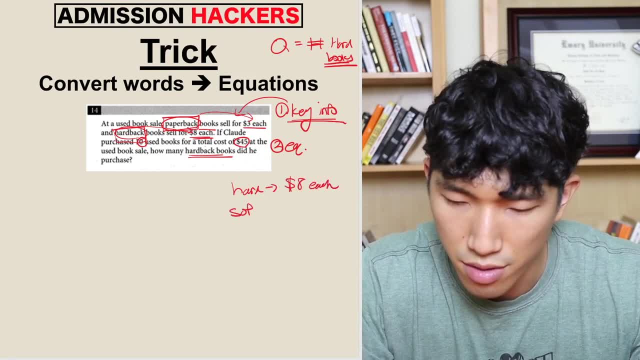 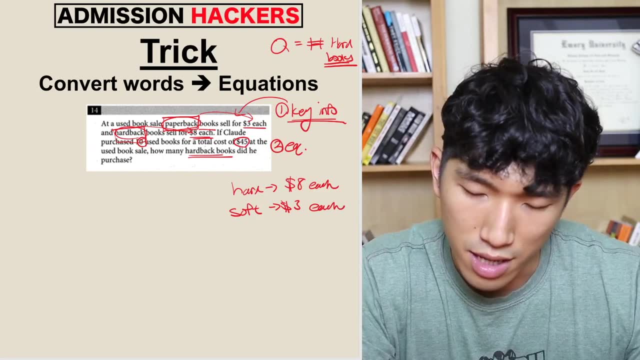 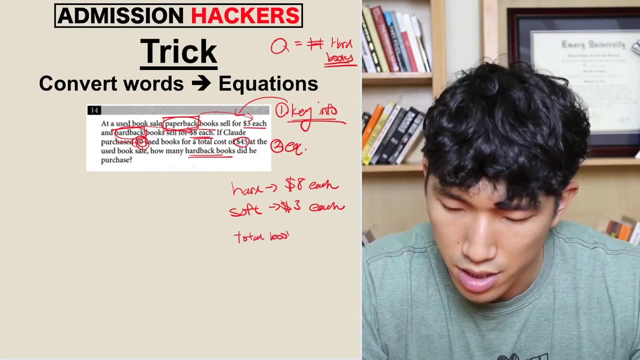 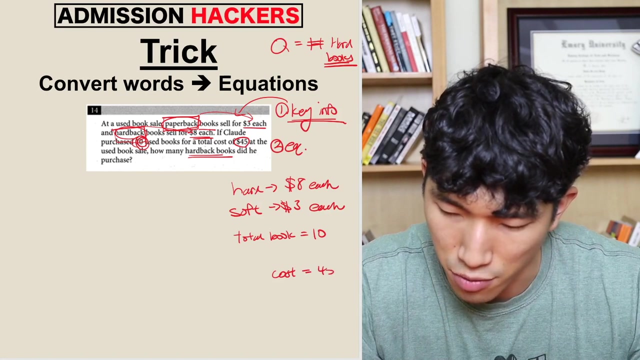 And soft is going to be $3 each, Okay, And another thing that the question tell us is that the person purchased 10 books total, So we know that total book is going to be 10, right, And the total cost is going to be $45, right. And based on this key information, what we're going to do is we're going 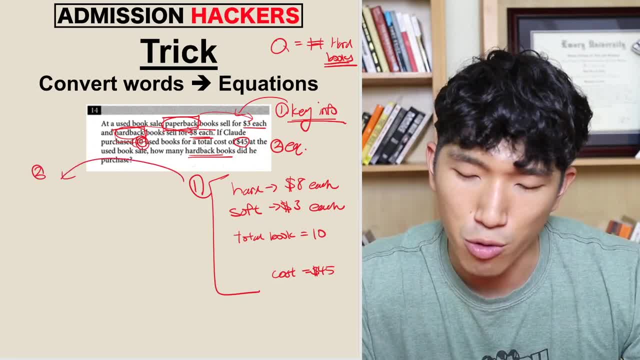 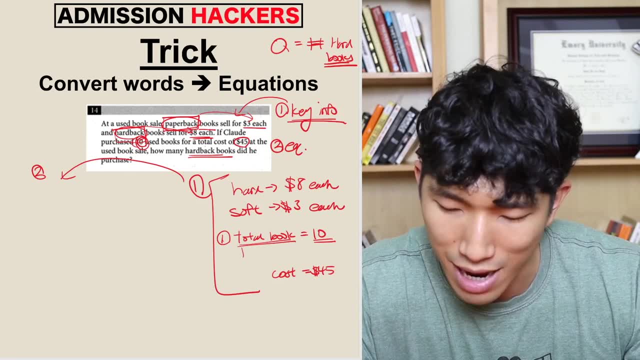 to create a search engine. So we're going to create a search engine And we're going to create a create equations. Okay, So our first equation is going to be based on the total number of books, and the total number of books is going to be 10.. And we know that total number of books is made out. 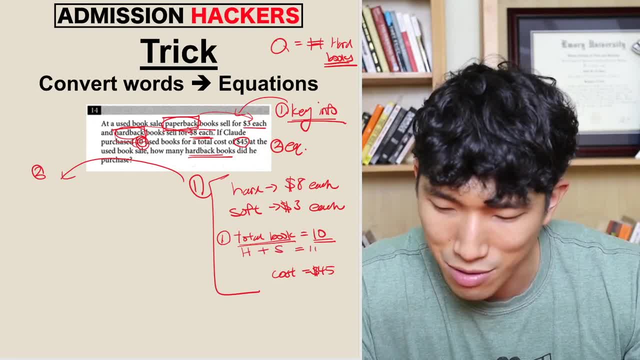 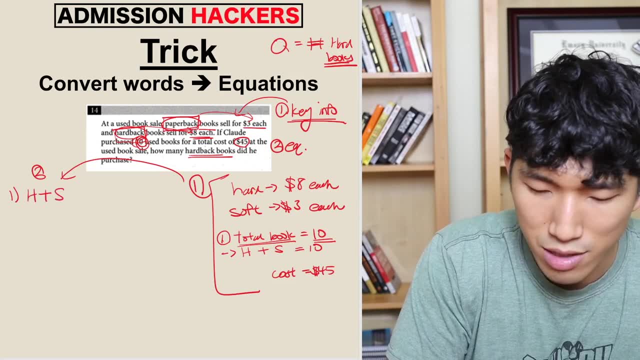 of hard books plus soft books, right? And that's going to equal 10.. And that's going to be your first equation, right there? right? So our equation number one is going to be H plus S, which is number of hard books plus number of soft books, And that's going to equal 10.. And the second: 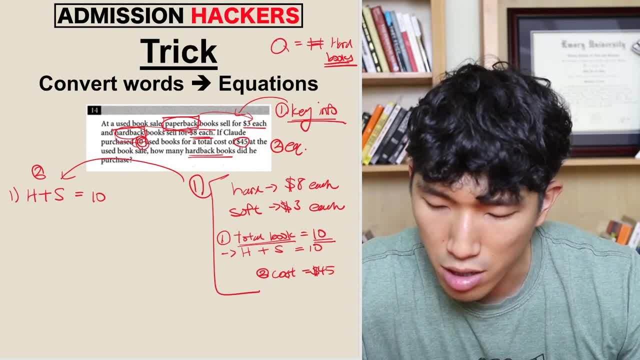 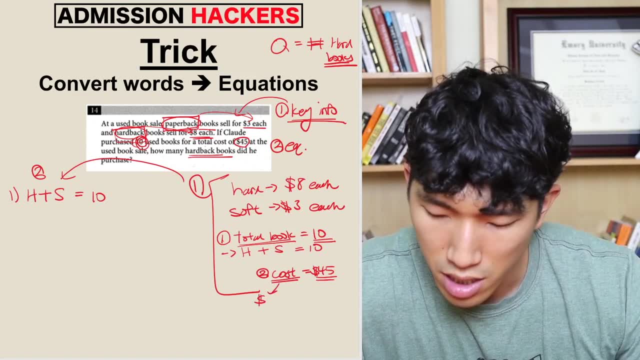 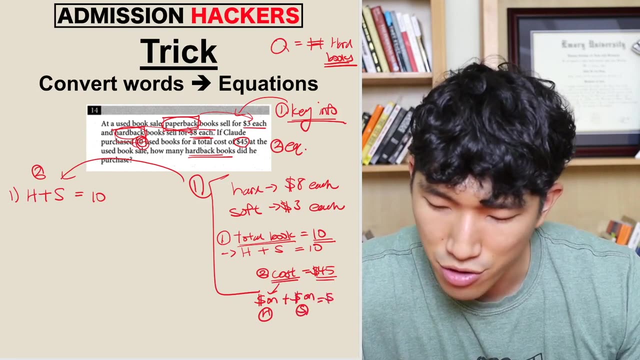 equation is going to come from our cost. Okay, So what we know is that the total cost, the total money that they spent on the book, was $45.. So total cost comes from money on hard books plus money on soft books, right, And if you add those two monies up, you get the total cost, which is: 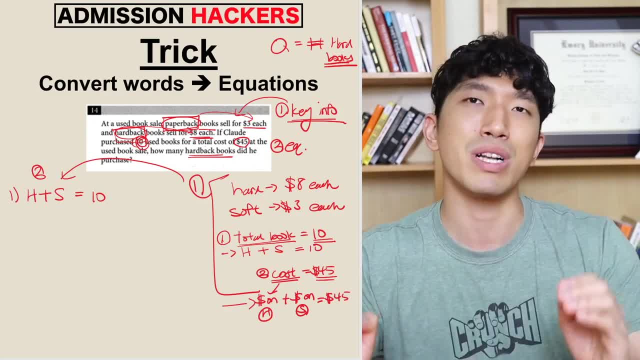 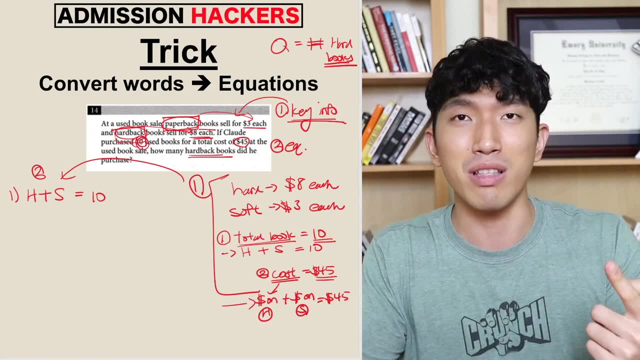 $45.. So how can we find out exactly how much money was spent on hard books? That's really simple. You just multiply the number of hard books that you bought by how many you bought. If you multiply those two things together, you can find out how much it, how much, you spent on hard books. 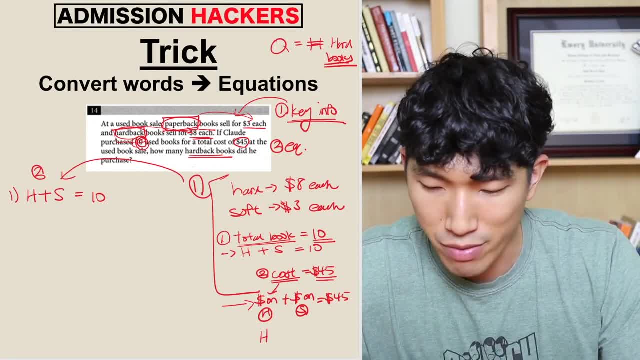 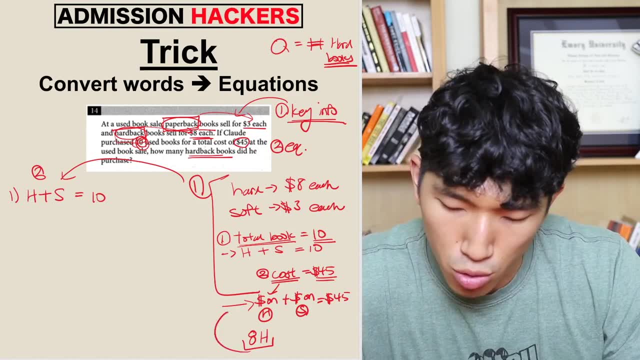 So how many hard books did we buy? We bought H books. We don't know how many we bought and how much do they cost each. It's going to be $8 each, And if you do eight H, that's going to give you the total money spent on hard books And you can do the similar for soft books. It's going 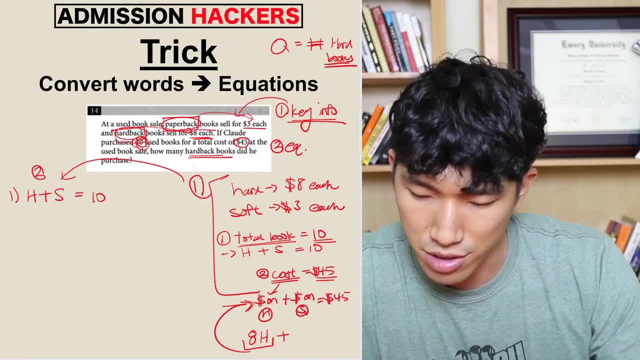 to be: how much is the book? Um, how much is the soft book? It's going to be $3.. And how many did you buy? You bought S soft books, And if you do that, it's going to end up with $45.. equation is going to come from our cost. Okay, So our first equation is going to be: 지inyi Jag giorno. We know there's an American highway range in the United States and there's going to be a basis Paraíso. Damn Hard Bang. 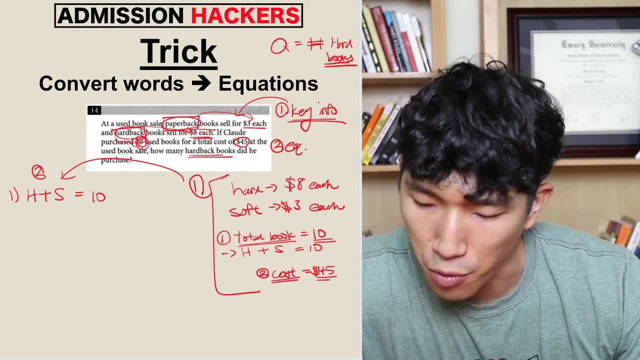 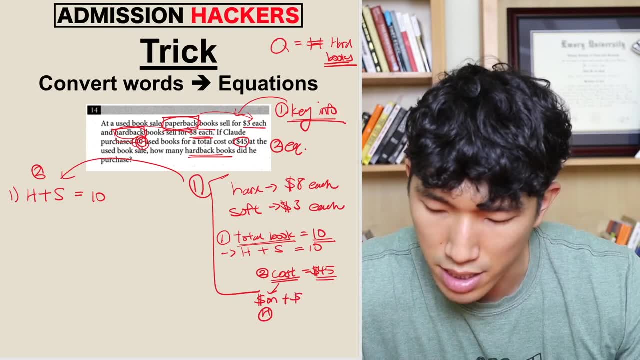 product lower side of the Сер cis buses, higher side of the Center. for period of time This can be, is that the total cost, the total money that they spent on the book, was 45, so the total cost comes from money on hard books plus money on soft books. right, and if you add those two monies up you get. 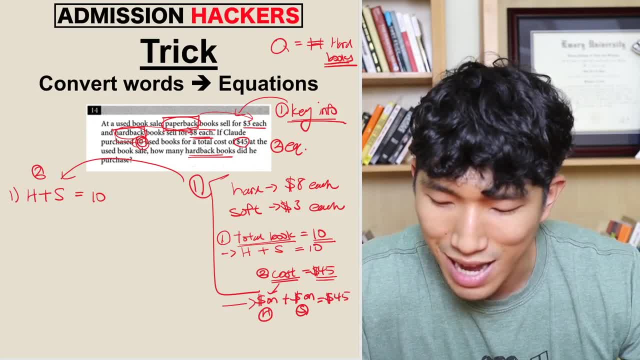 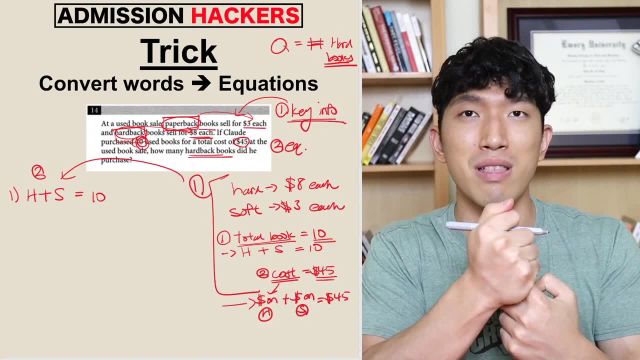 the total cost, which is 45. so how can we find out exactly how much money was spent on hard books? that's really simple. you just multiply the number of hard books that you bought by how many you bought. if you multiplied those two things together, you can find out how much it how much. 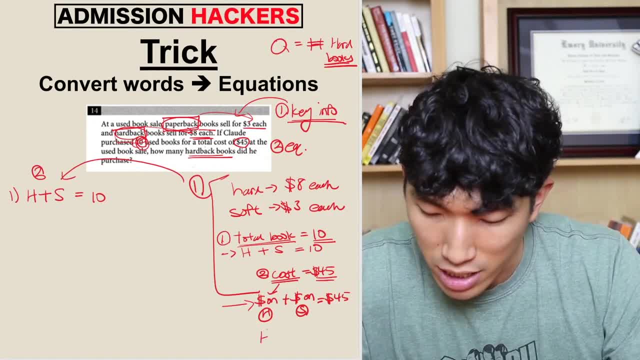 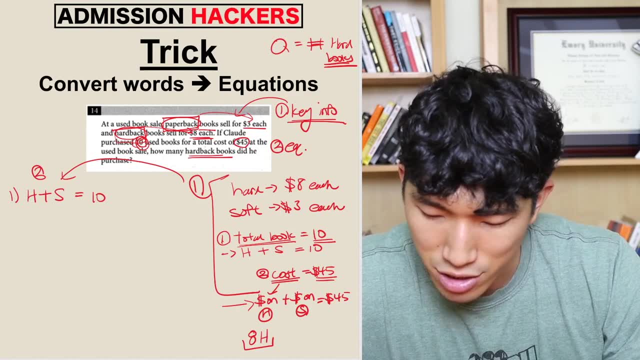 you spent on hard books. so how many hard books did we buy? we bought h books. we don't know how many we bought and how much do they cost each. it's going to be eight dollars each and if you do eight h, that's going to give you the total money spent on hard books and you can do the. 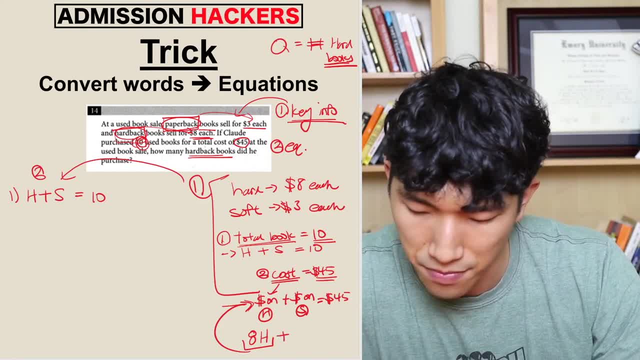 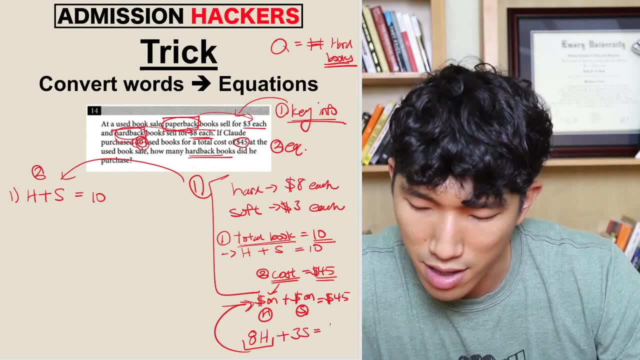 similar for soft books. it's going to be: how much is the book? um, how much is the soft book? it's going to be three dollars. and how many did you buy? you bought s soft book, and if you do that, it's going to end up with. 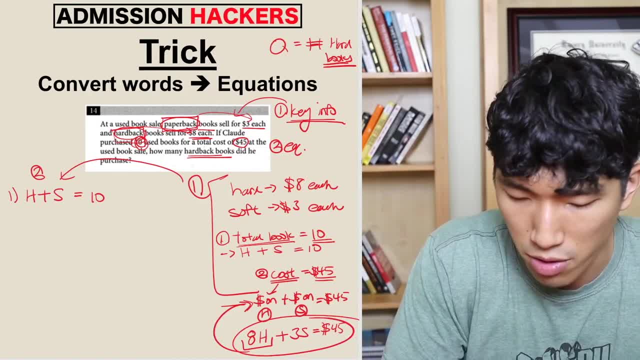 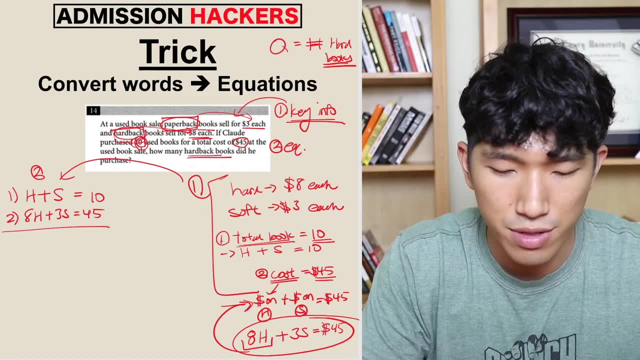 $45.. And that's going to be your second equation. So what we do is we put it right there: 8H plus 3S is going to equal 45. And now we're going to use these two equations to find out exactly how. 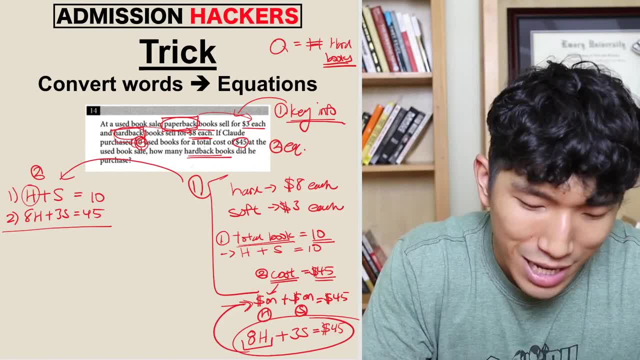 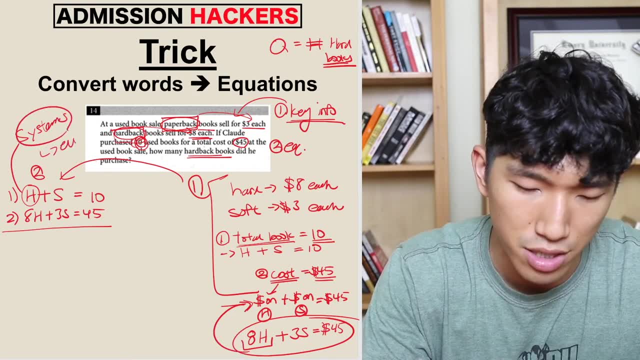 many hardbooks that we bought. Okay, So what we're looking for is H. So we're going to use systems of equations to find out exactly what H is, And we're going to use elimination. Okay, If you're not sure why we're using elimination here, go back to a systems lecture. There's going to be a link. 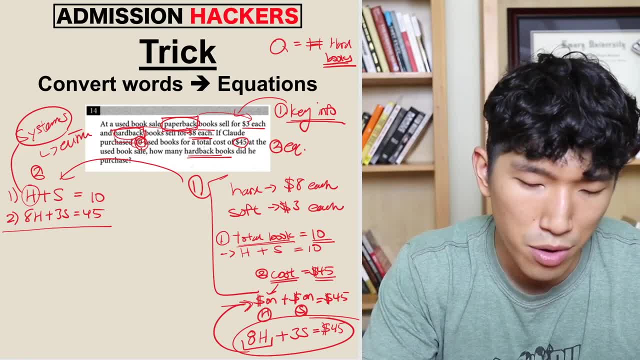 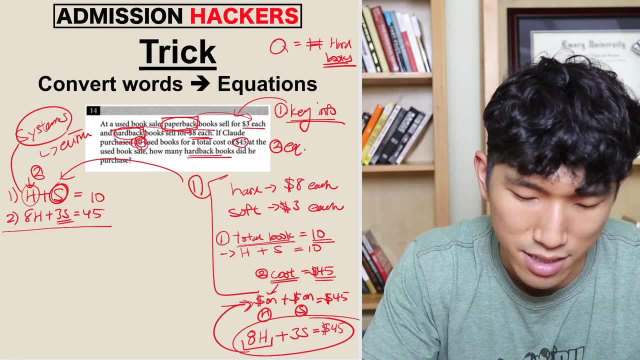 right there, It's going to outline exactly everything you need to know. Since what we're looking for is H, we're going to try to eliminate S And how we can do that. multiply the top equation by 3.. That will match up the S's, So it's going to become 3H plus 3S is equal to 30.. Okay, 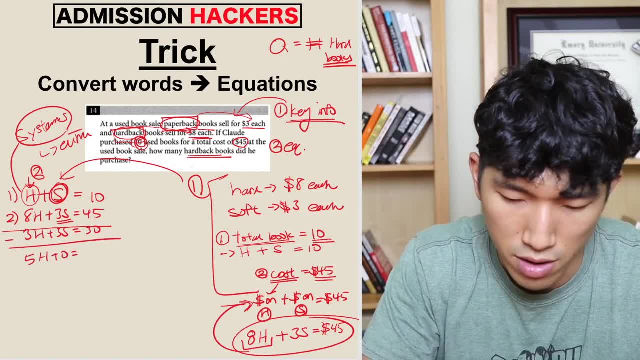 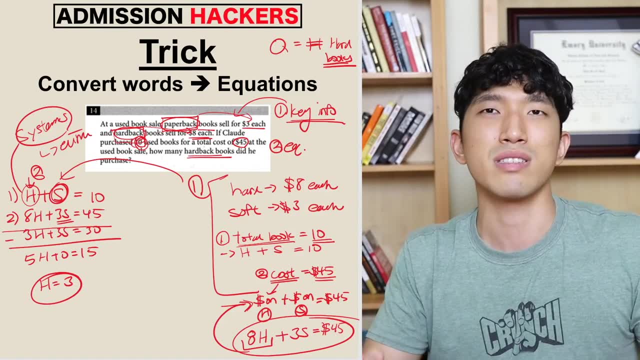 And if you subtract the whole thing, you end up with: 5H plus 0 is equal to 15.. You get that H is equal to 3.. Okay, That means we bought three hardbooks total. Okay, So it's actually really. 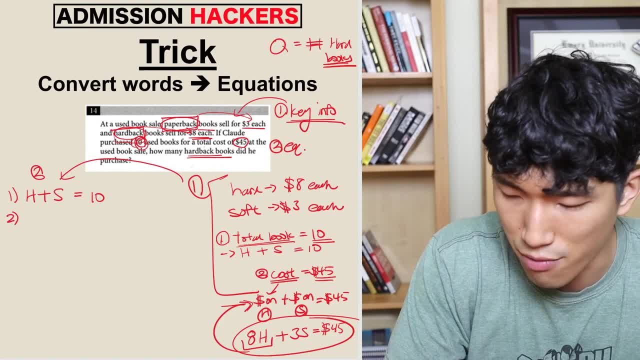 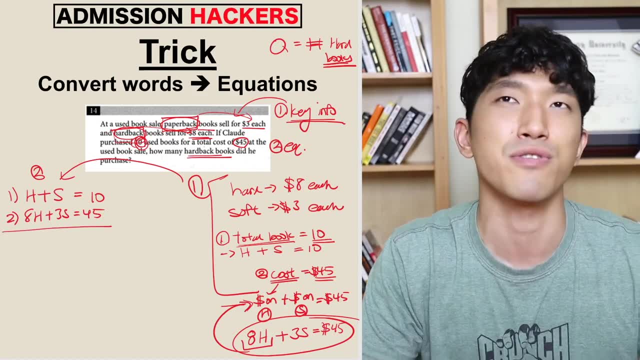 And that's going to be your second equation. So what we do is we put it right there: Eight H plus three S is going to equal 45. And now we're going to use these two equations to find out exactly how many hard books that we bought. Okay, So what we're looking for is H, So we're. 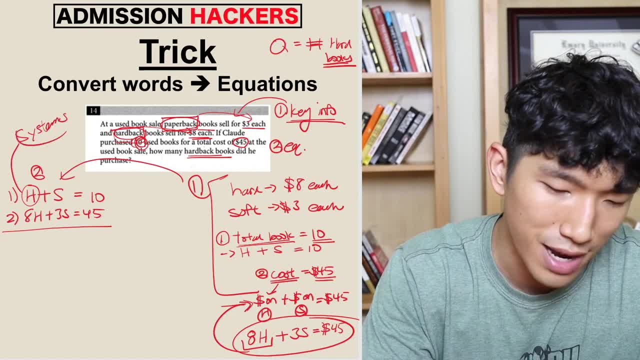 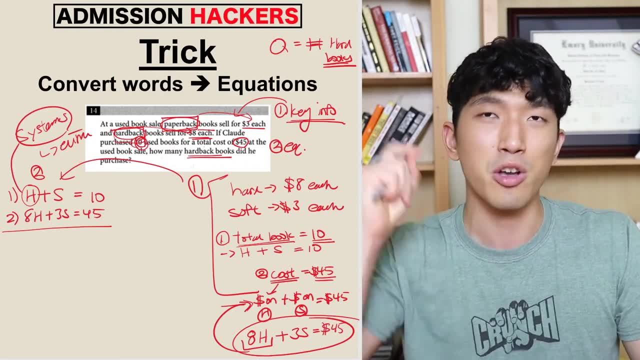 going to use systems of equations to find out exactly what H is, And we're going to use elimination. Okay, If you're not sure why we're using elimination here, go back to a systems lecture. There's going to be a link right there. It's going to outline: 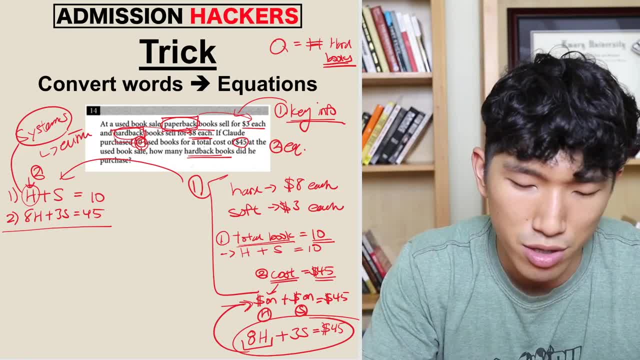 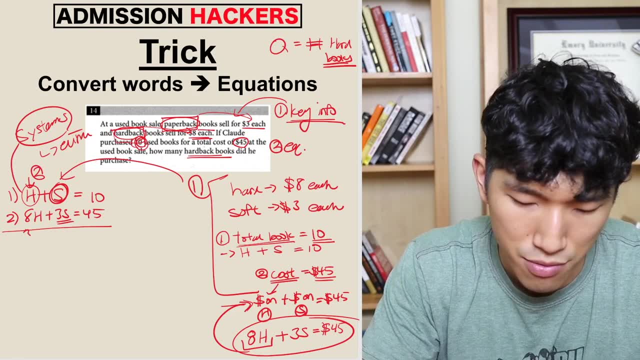 exactly everything you need to know. Since what we're looking for is H, we're going to try to eliminate S, and how we can do that. Multiply the top equation by three. that will match up the S's, So it's going to become three. H plus three S is equal to 30.. Okay, And if you subtract the whole, 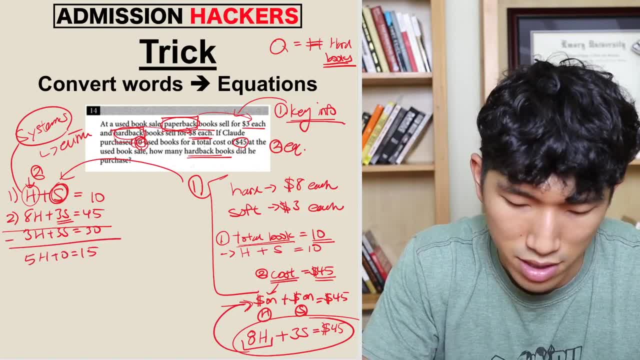 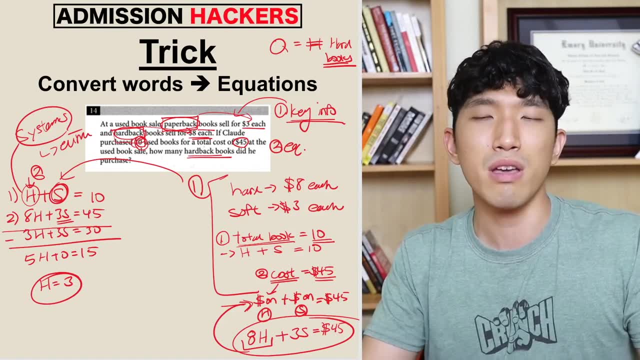 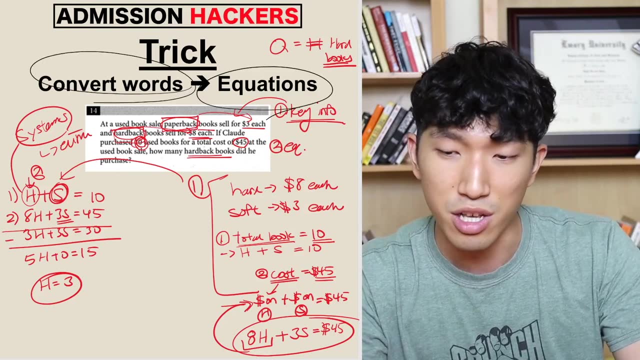 thing you end up with: five H plus zero is equal to 15.. You get that H is equal to three. Okay, That means we bought three hard books total, Okay. So it's actually really simple. All you have to do is go back into equations, And to do that you need two things. You first have to get key. 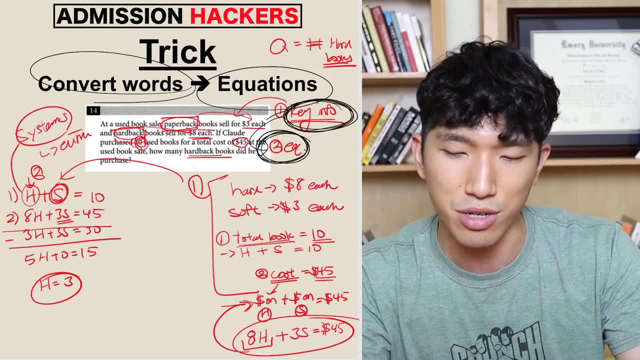 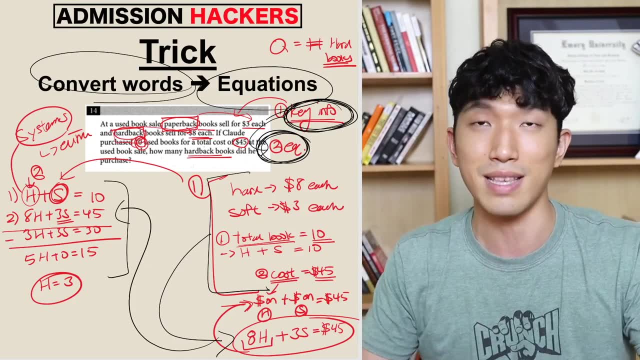 informations And based on the key information, you can make up this equation. Okay, So key information is here and equations look like that here, And you use that to solve and find the answer. Let's go to the second one. This one's actually going to be similar to the first one. 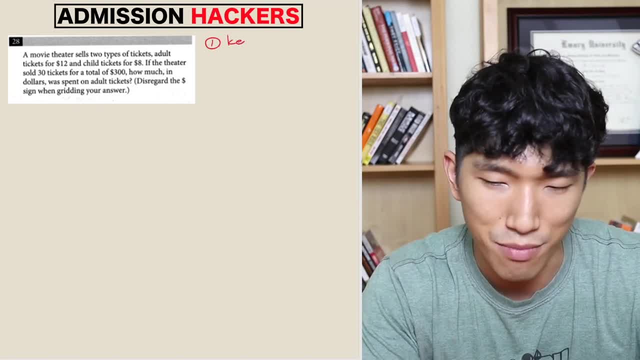 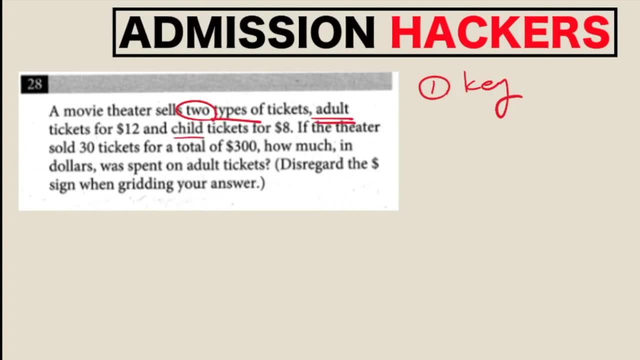 but let's try it out again. So the first thing we're going to do is identify the key information, right? So let's read the question. A movie theater sells two types of tickets. Okay, And there's going to be a adult ticket and there's going to be a child's ticket. 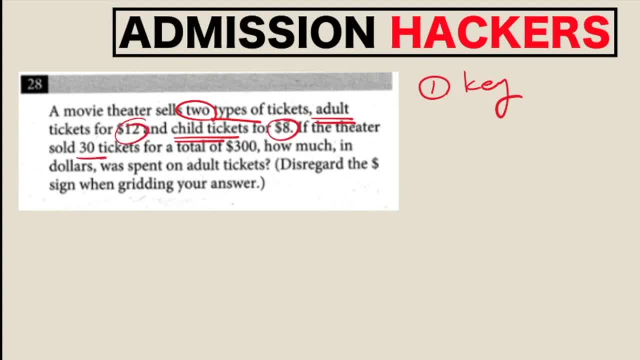 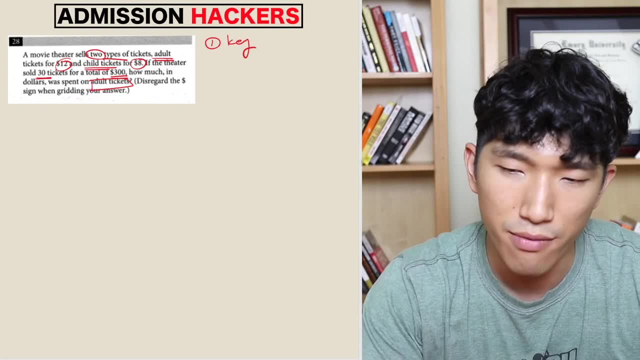 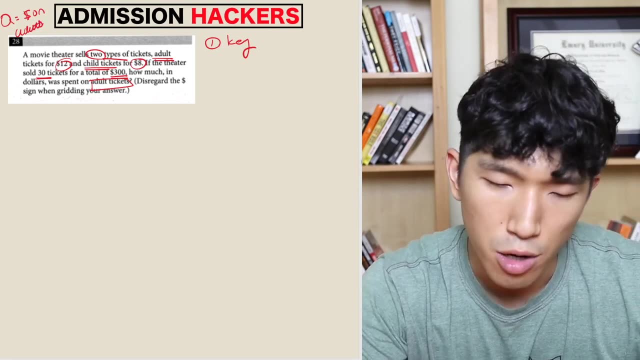 Adult is $12.. Child is $8.. If the theater sold 30 tickets for a total money of $300, how much in dollars was spent on adult tickets? Okay, So what are we looking for? The question is: money on adults. Okay, That's what we're looking for. So identify the key information. 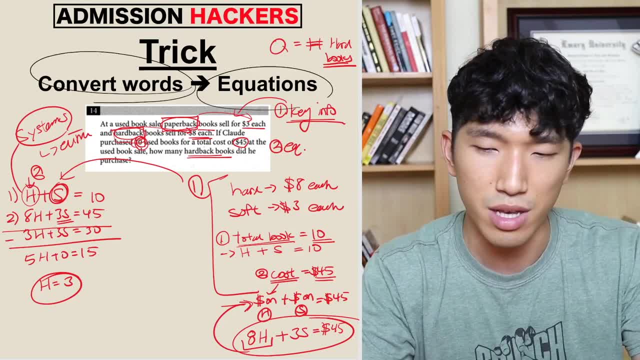 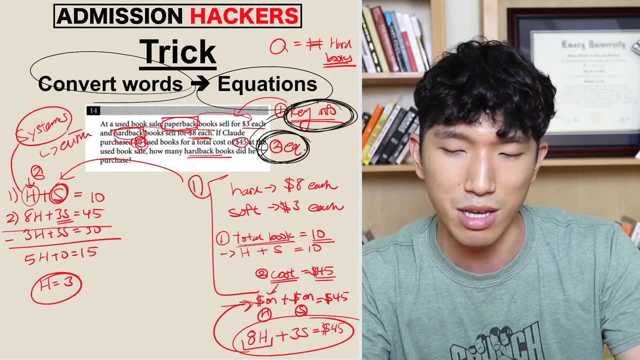 simple. All you have to do is just Convert words into equations, And to do that you need two things. You first have to get key information, And based on the key information you can make up this equation. Okay, So key. 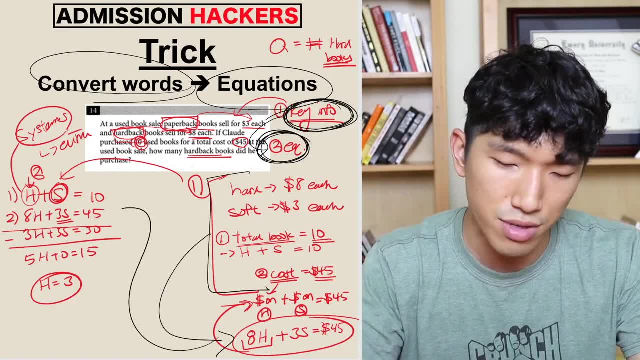 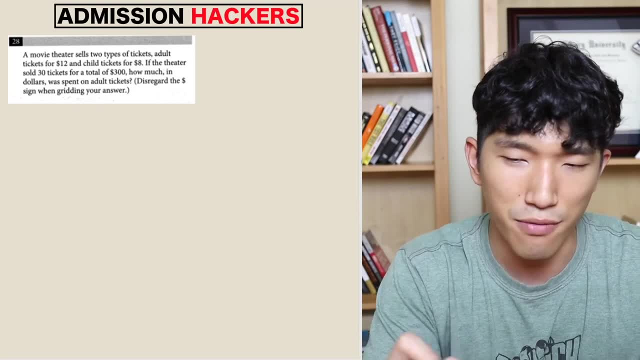 information is here and equations look like that here And you use that to solve and find the answer. Let's go to the second one. This one's actually going to be similar to the first one, but let's try it out again. So the first thing we're going to do is identify the key information. 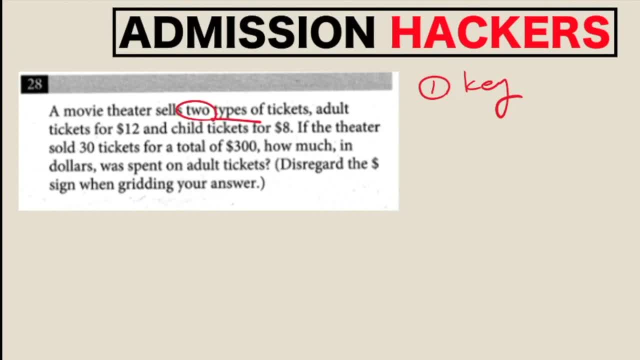 Right, So let's read the question. A movie theater sells two types of tickets. Okay, And there's going to be a child's ticket. Adult is $12.. Child is $8.. If the theater sold 30 tickets for a total money. 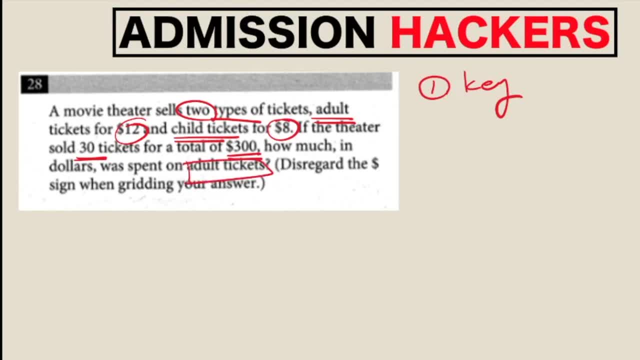 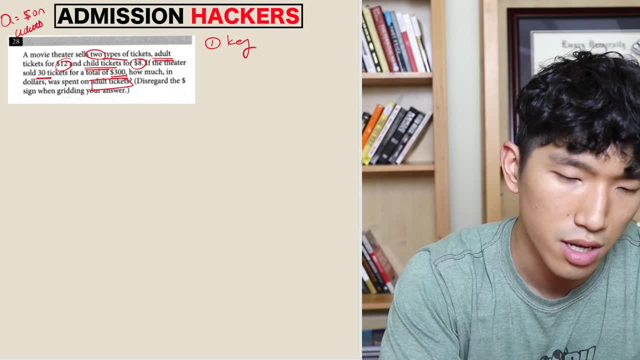 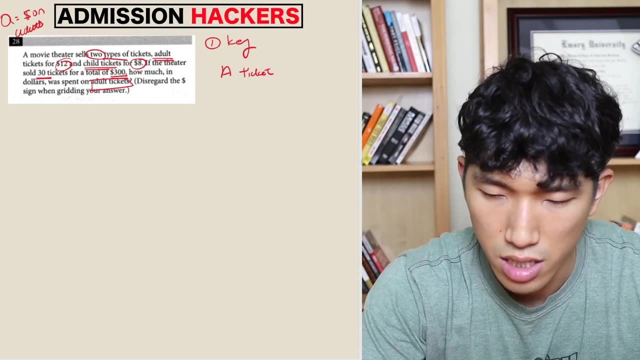 of $300, how much in dollars was spent on adult tickets? Okay, So what are we looking for? The question is: money on adults. Okay, That's what we're looking for. So identify the key information. We know that adult tickets- It's going to be adult ticket- It's going to be $12.. And a child's? 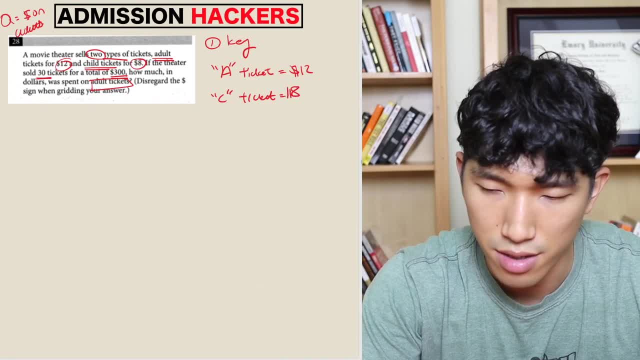 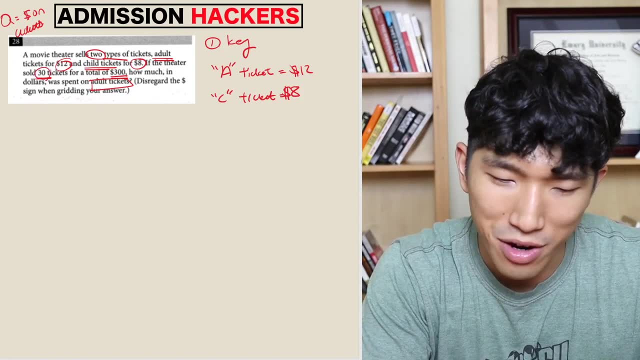 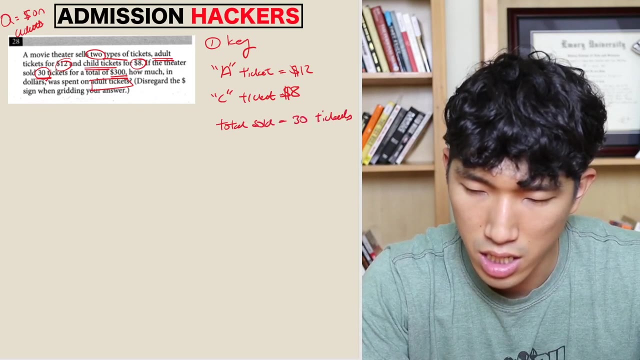 ticket is going to be $8.. $8. That's a terrible dollar. It's going to be $8.. Right, And what we know is that they sold total of 30 tickets, Right, So total sold is going to be 30 tickets And total money from 30. 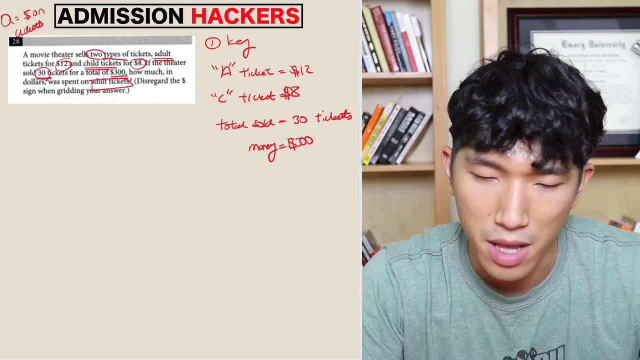 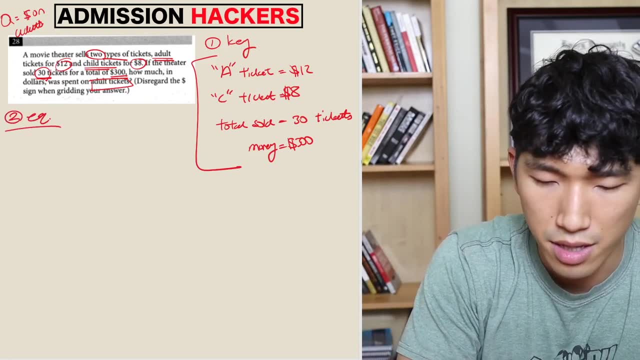 ticket sales is going to be $300.. Right, So, based on that, we are going to now make an equation out of it. Okay, So the second step is equation. So what we know is: total number of tickets sold is going to be 30 tickets And total sold is made. 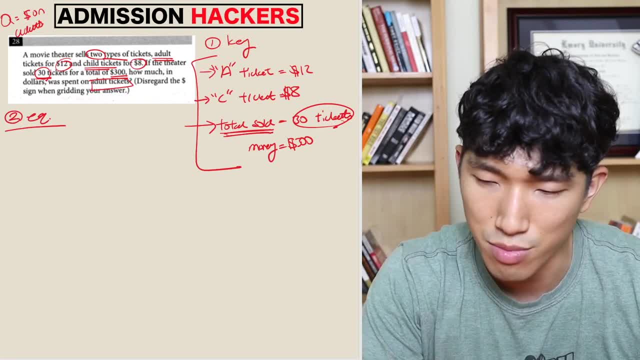 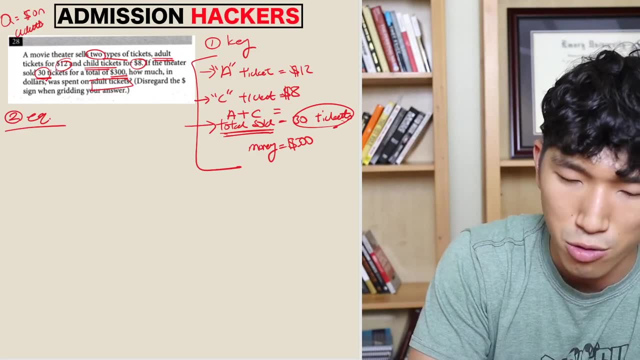 up by number of adult tickets and number of children's tickets, Which means total sold is going to be same as adult plus children's tickets And that's going to equal 30 tickets, Which means your equation is going to be: A plus C is going to equal 30. Because A is the number of the adult. 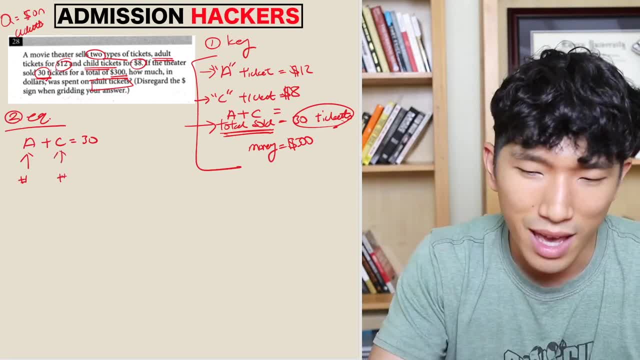 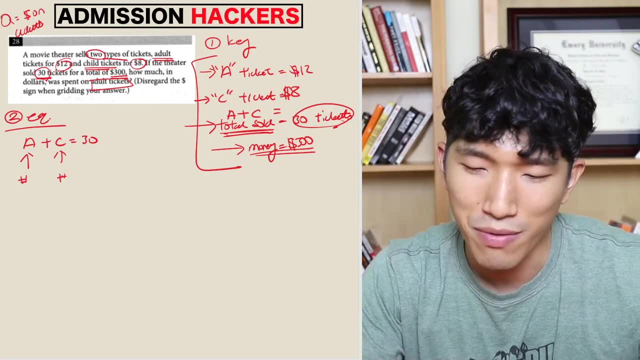 and C is the number of children's tickets sold Right, And the second equation that we can get is the amount of money generated or the amount of money generated Right. So how do we find the left side? Well, we know that money generated is made up two parts. It's going to be money. 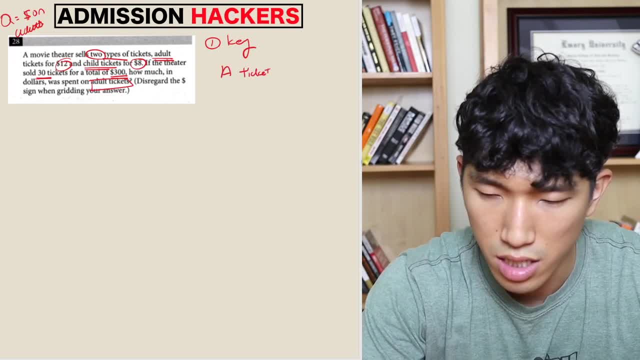 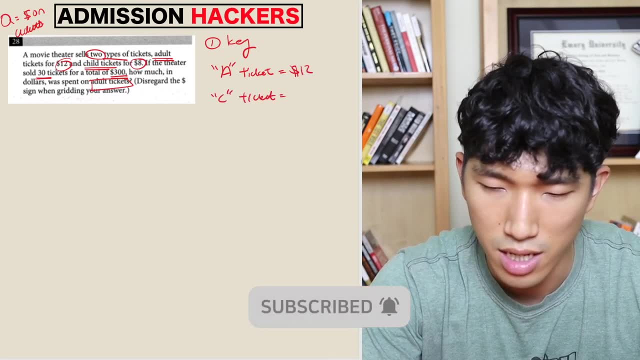 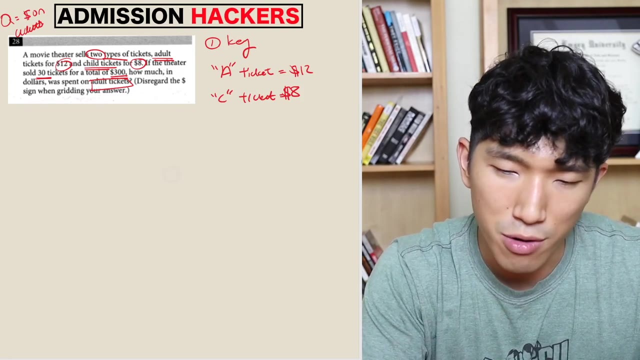 We know that adult tickets- it's going to be adult ticket- It's going to be $12.. And a child's ticket is going to be $8.. $8. That's a terrible dollar. It's going to be $8, right. And what we know is that they sold. 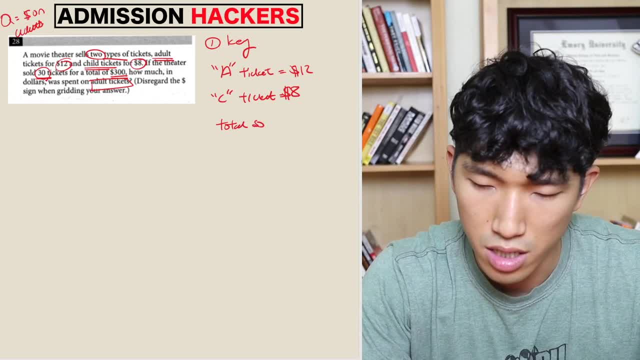 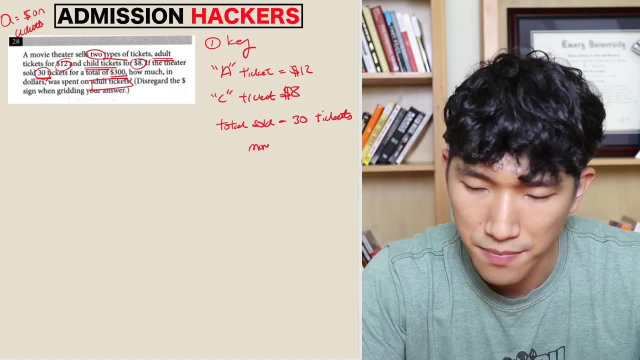 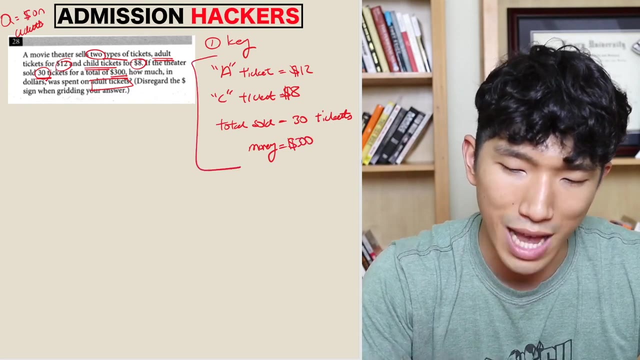 total of 30 tickets. right, So total sold is going to be 30 tickets and total money from 30 ticket sales is going to be $300, right? So based on that, we are going to now make an equation out of it. Okay, So the second step is equations. 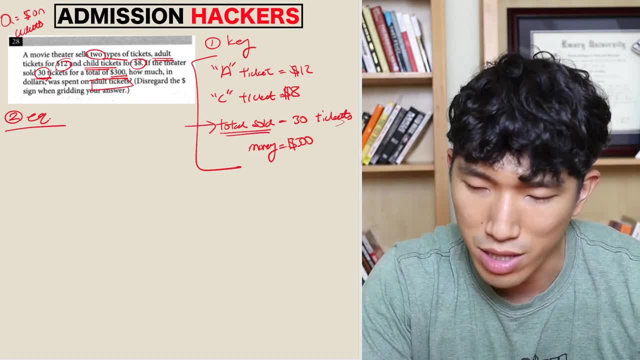 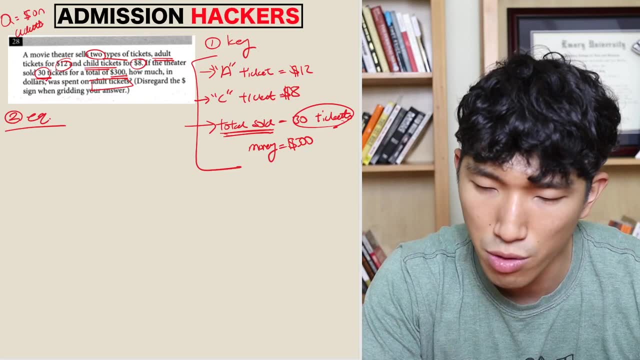 So what we know is total number of tickets sold is going to be 30 tickets, and total sold is made up by number of adult tickets and number of children's tickets, which means total sold is going to be same as adult plus children's tickets, And that's going to equal 30 tickets, which means 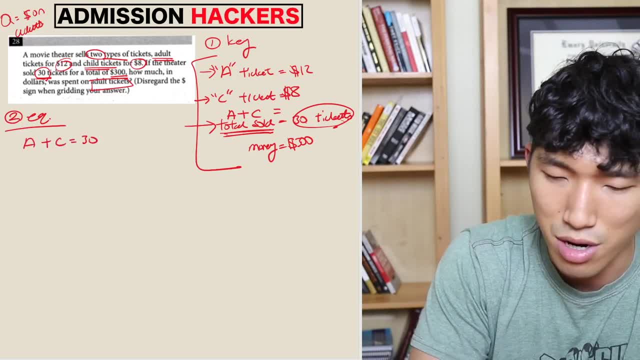 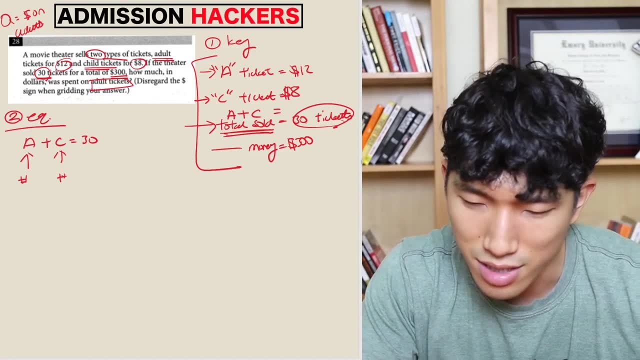 your equation is going to be: A plus C is going to equal 30, because A is the number of the adult and C is the number of children's tickets sold right. And the second equation that we can get is from the number of money generated. 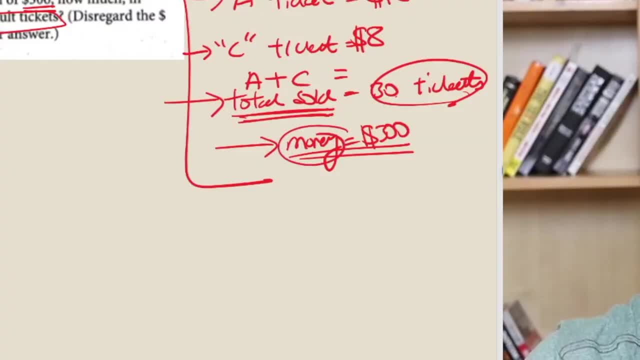 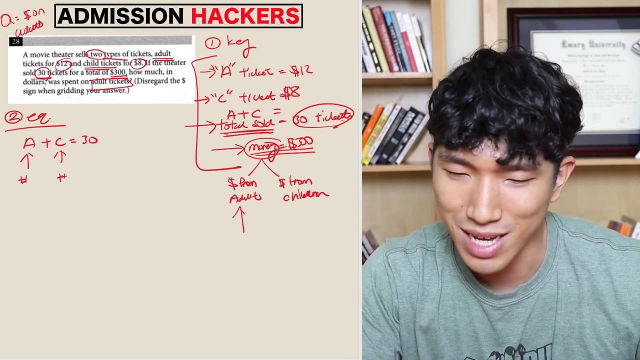 I don't have money generated, right. So how do we find the left side? Well, we know that money generated is made up two parts. It's going to be money from adults ticket sales and money from children ticket sales, right? So how do we find out the money from adult ticket sales? You just 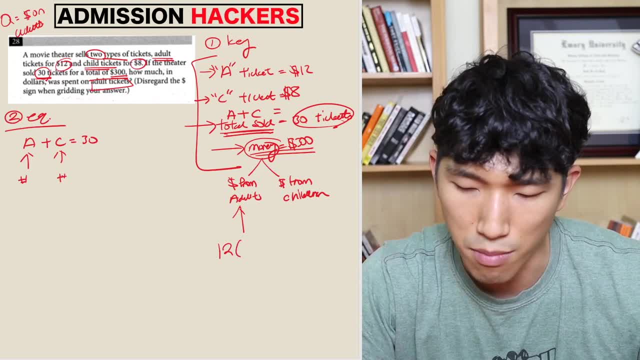 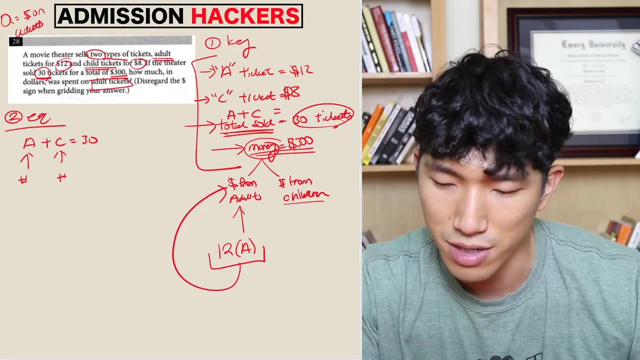 multiply the cost, which is $12, by the number of adults tickets sold. That will give you a number of money generated from adults tickets. And next thing you can do is for the same thing for children tickets. it's going to be eight times C and that's going to give you the money generated from. 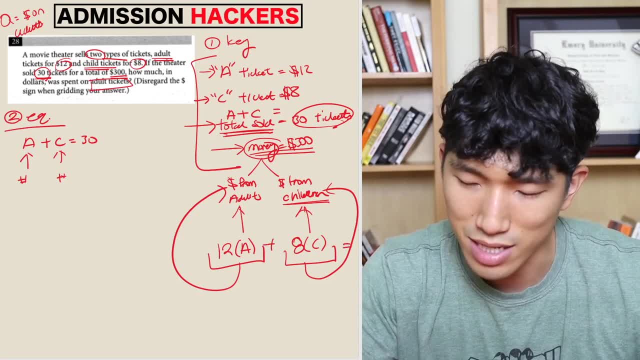 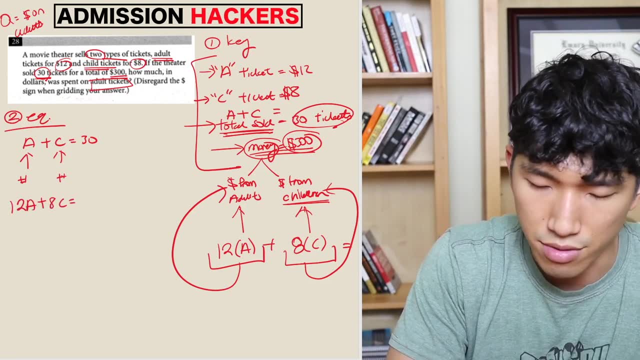 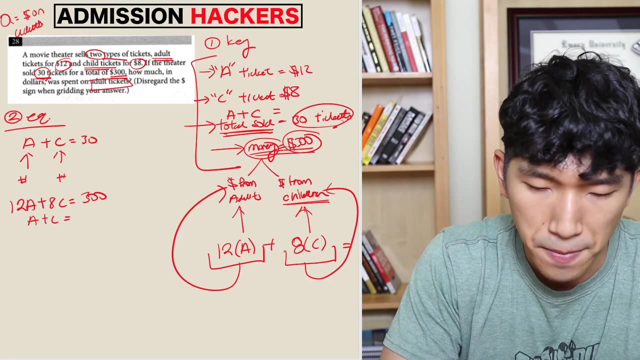 children's tickets. So that is going to the sum of it is going to equal to what It's going to equal: 300, which means 12 A plus eight C is equal to 300.. Okay, And now that we got two equations, 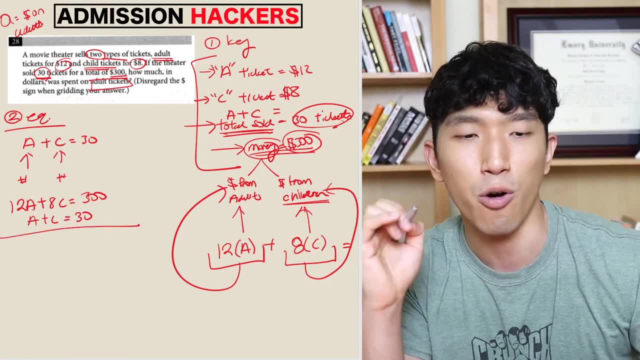 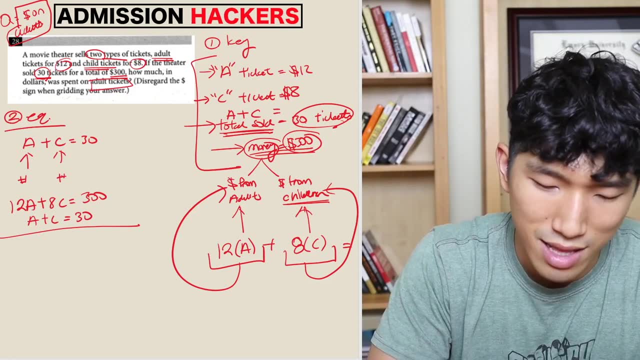 what we can do is we can use substitution or elimination to find out what we have to find. And what we have to find out is how much money was spent on adult tickets and how. what represents that? it's going to be 12 A, because 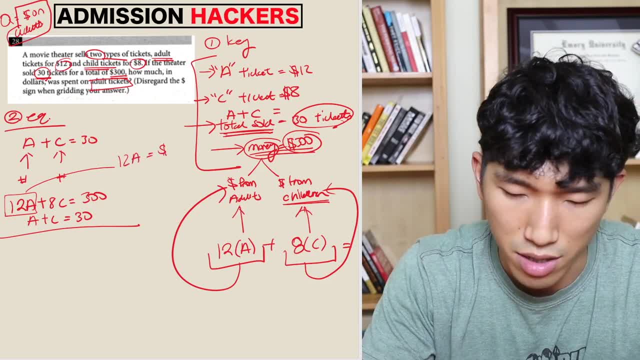 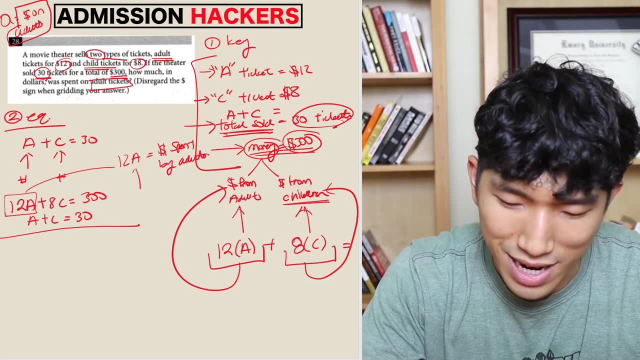 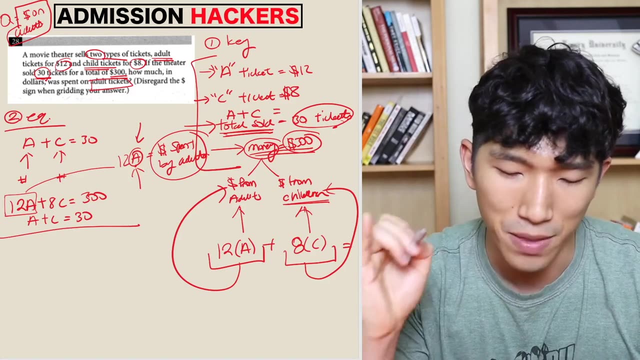 12 times A is going to give you money spent on money spent by adults, right? So what we need to do is find out what A is and plug it in, and then we can find out the money spent by adults. Okay, So what we need to do is find A. and how can we do that? We can do that by getting rid of the C. 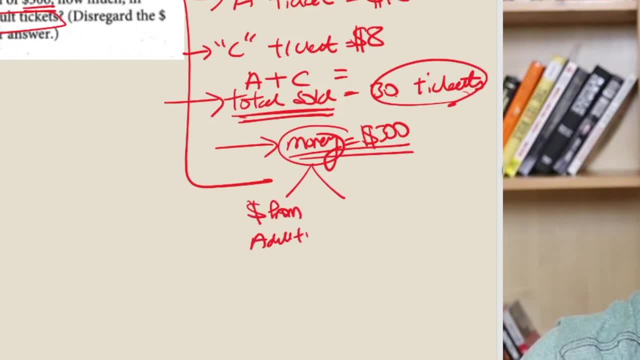 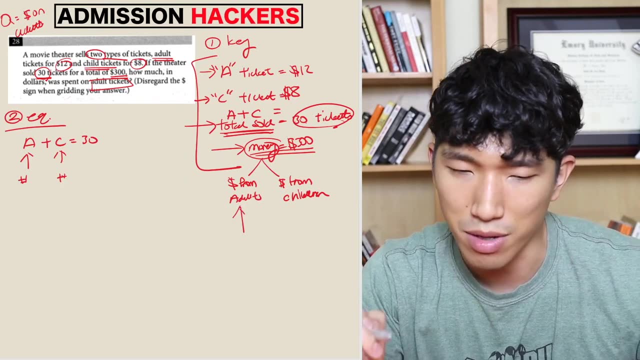 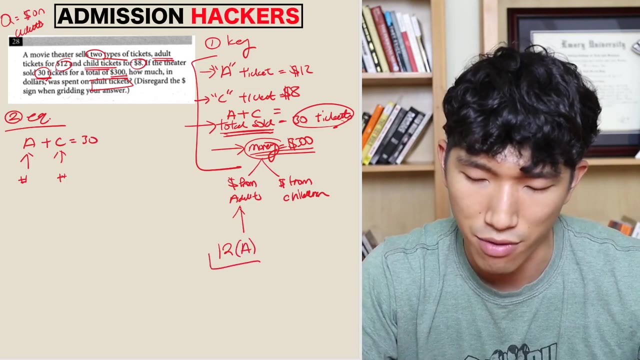 from adults ticket sales and money from children ticket sales. Right, So how do we find out the money from adult ticket sales? You just multiply the cost, which is $12, by the number of adults tickets sold. That will give you a number of money generated from adults tickets And next. 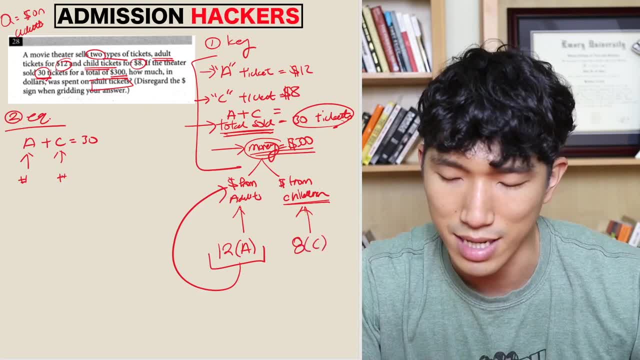 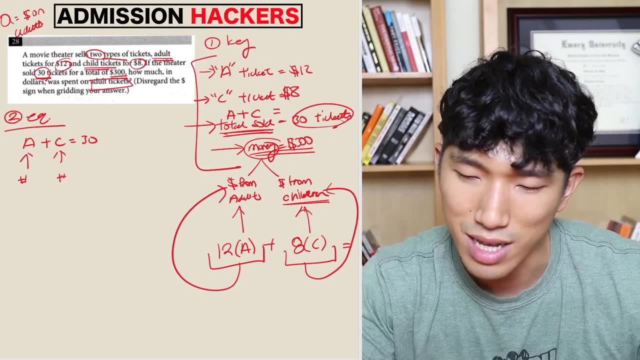 we're going to do the same thing for children. It's going to be eight times C And that's going to give you the money generated from children's tickets. So that is going to the sum of it is going to equal to what It's going to equal 300. Which means 12A plus eight C is equal to. 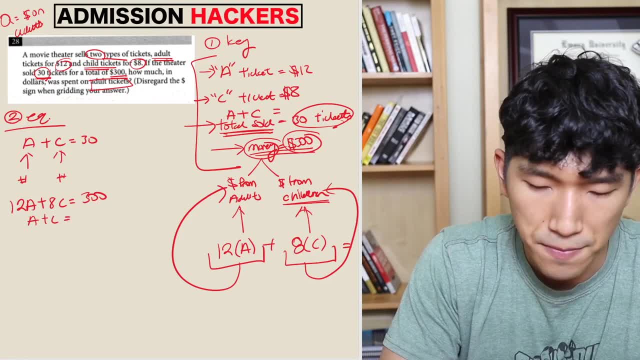 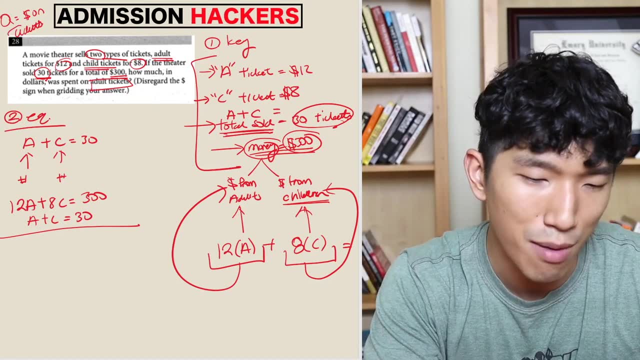 300.. Okay, And now that we got two equations, what we can do is we can use substitution or elimination to find out what we have to find. And what we have to find out is how much money was spent on adult tickets and how. what represents that it's going to be 12A. 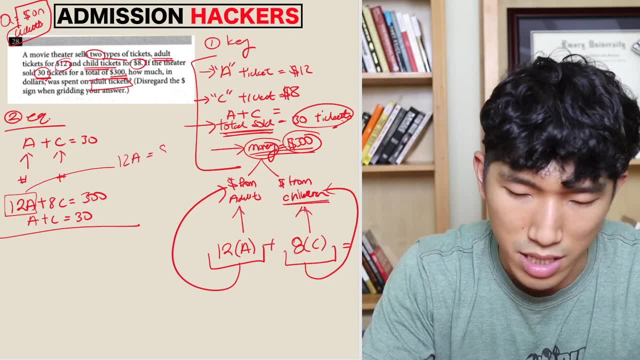 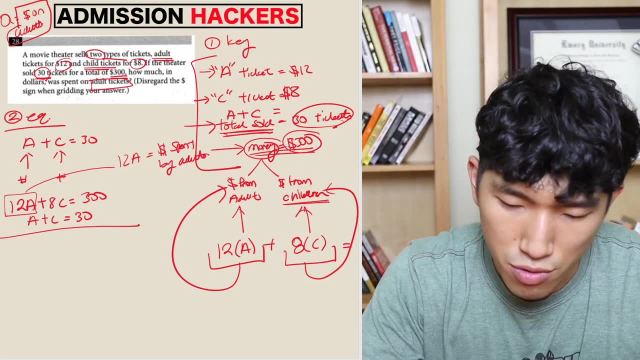 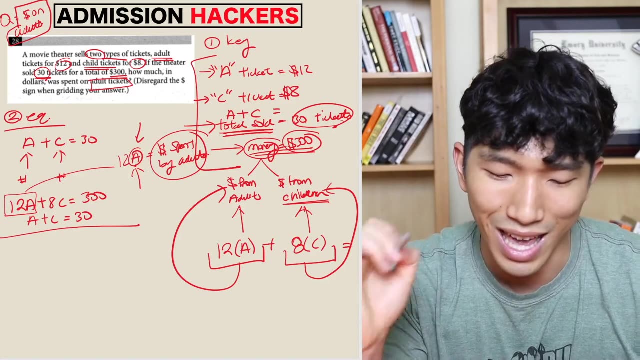 because 12 times A is going to give you money spent on money spent by adults, Right? So what we need to do is find out what A is and plug it in, and then we can find out the money spent by adults. Okay, So what we need to do is find A, and how can we do that? 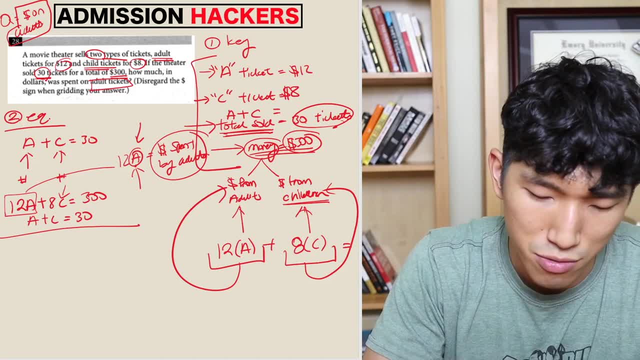 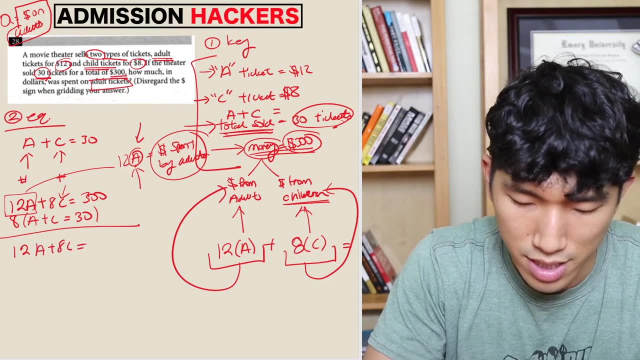 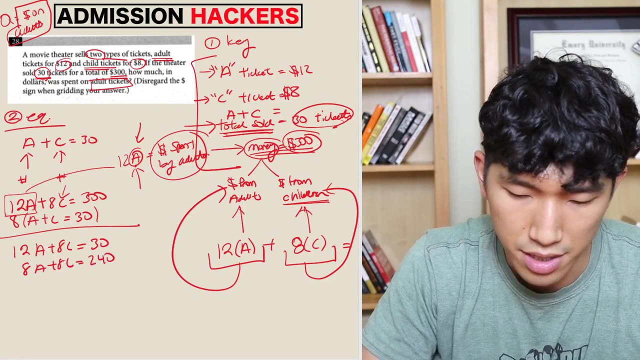 We can do that by getting rid of the C. So what we're going to do is multiply the bottom equation by eight so that our C's are matching up, So 12A- let me just write this down one more time- and multiply by eight. eight A plus eight C is going to equal to 40.. Okay, And what do we do? 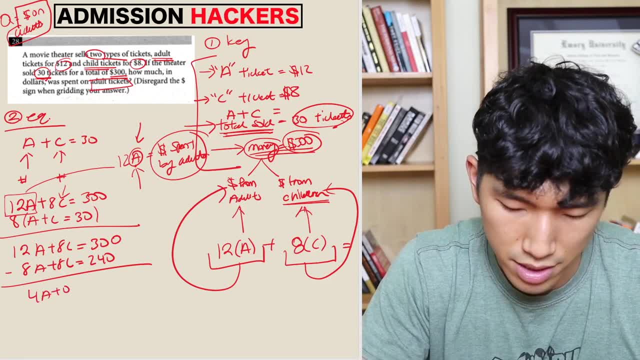 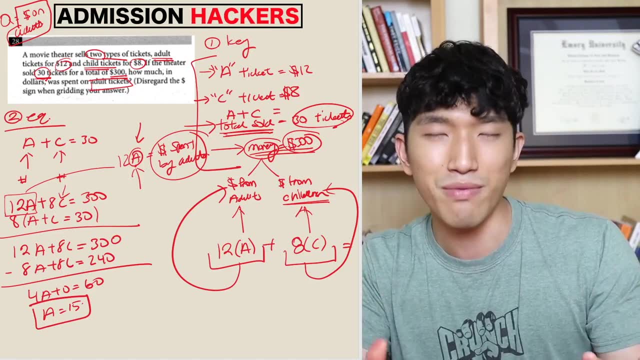 We subtracted and that will be four. A plus zero is equal to 60.. A is equal to 15.. Okay, That means we sold a total of 18 or 15 adult tickets. And with this, what do we do? We plug it. 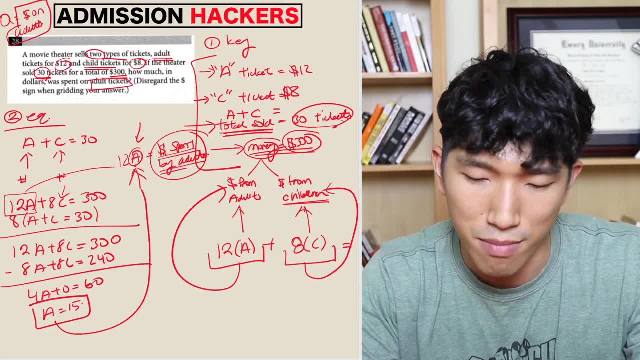 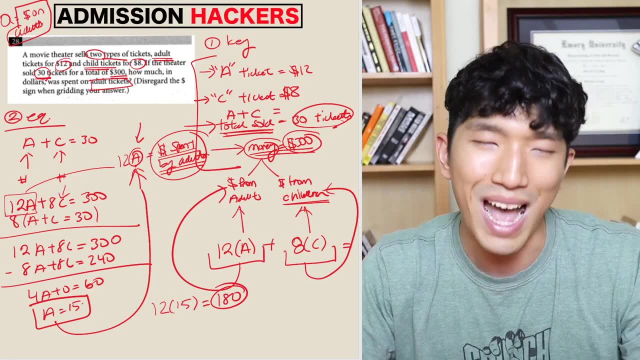 in to 12A and that should give us total money spent by the adults. So 12 times 15 is going to be 180, right, Yeah? So that is going to be your answer. How much did they spend on adults? They? 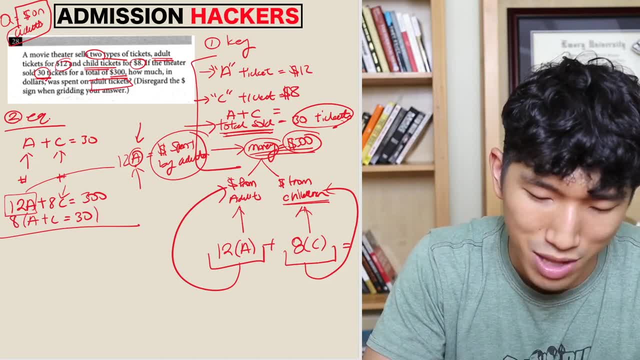 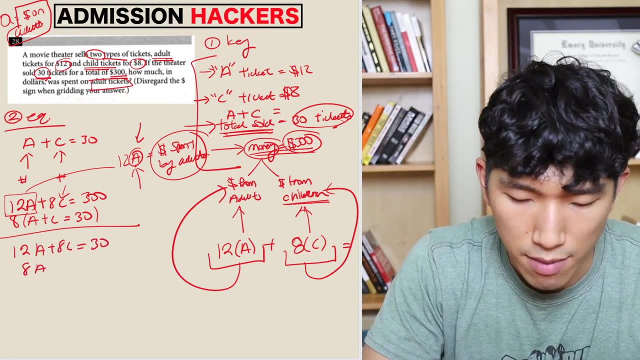 So what we're going to do is multiply the bottom equation by A, so that our C's are matching up. So 12 A- let me just write this down one more time- and multiply by eight. eight A plus eight C is going to equal to 40.. 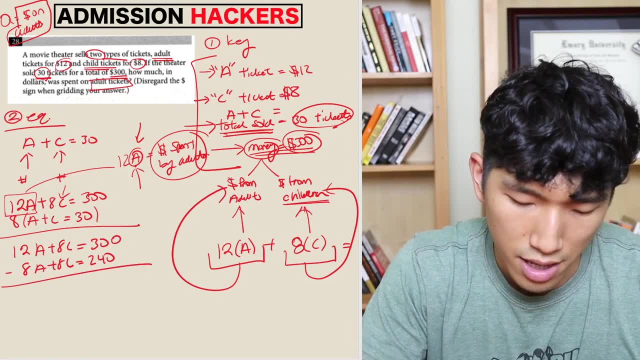 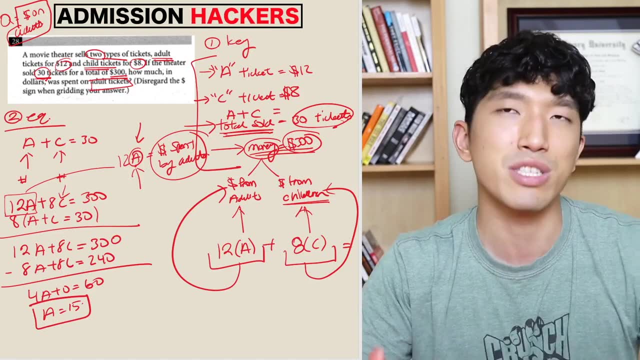 Okay, And what do we do? We subtracted, and that will be four: A plus zero is equal to 60. A is equal to 15.. Okay, That means we sold a total of 18 or 15 adult tickets. And with this, what do we? 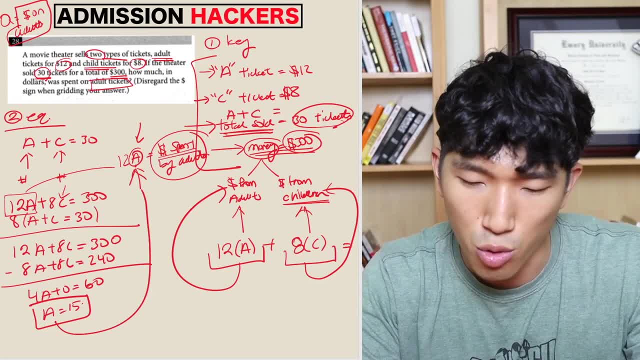 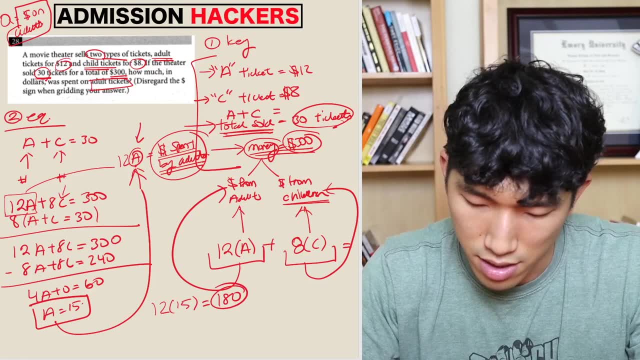 do We plug it in to 12 A, That should give us total money spent by the adults. So 12 times 15 is going to be 180, right, Yeah. So that is going to be your answer. How much did they spend on adults? They spent. 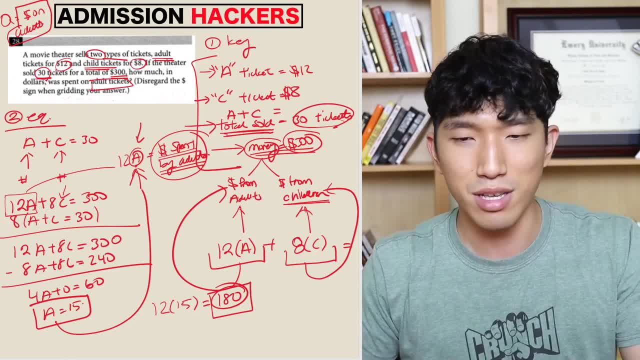 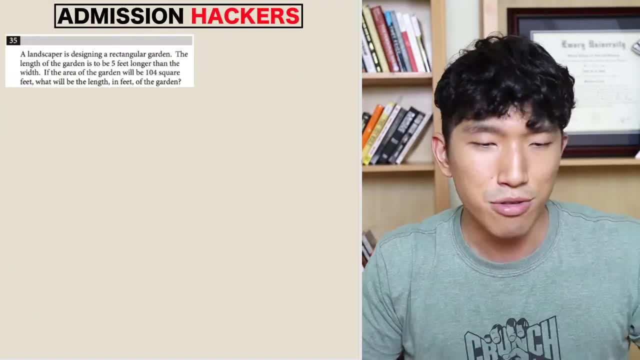 total of 180. Make sense. So the first thing you do is identify the key information And then with that you make two equations and you use systems to solve again. Let's go to the last one. A landscaper is designing a rectangular garden and the length of the garden is to be five feet longer. 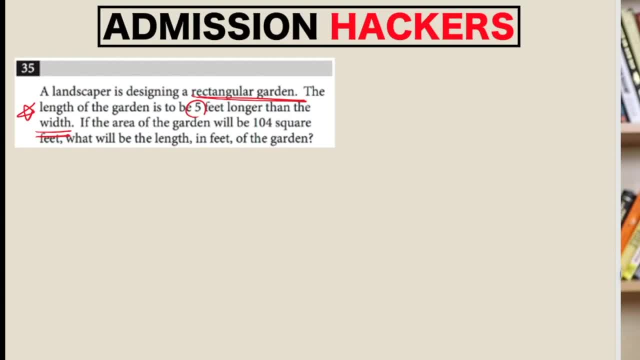 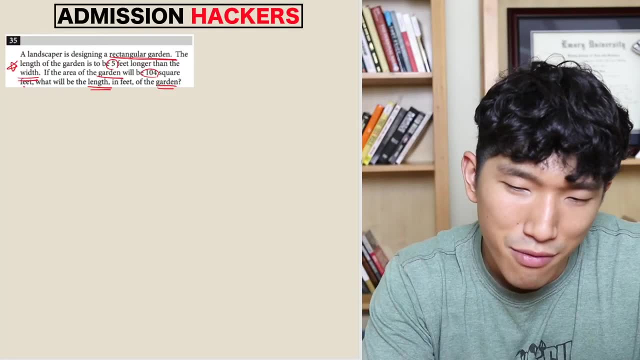 than the height of the garden. So the length of the garden is to be five feet longer than the height of the garden. the width: okay, that sounds pretty important. if the area of the garden will be 104 square feet, what will be the length and feet of the garden, right? so let's think about this, based on the 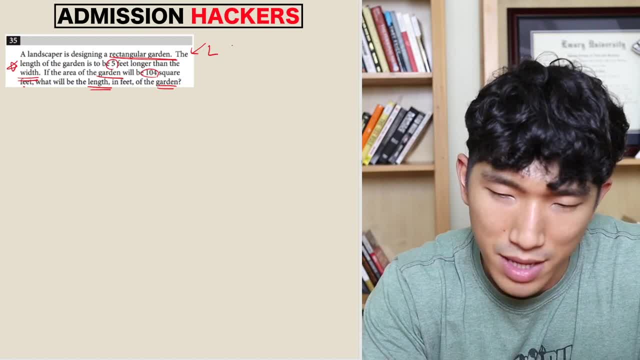 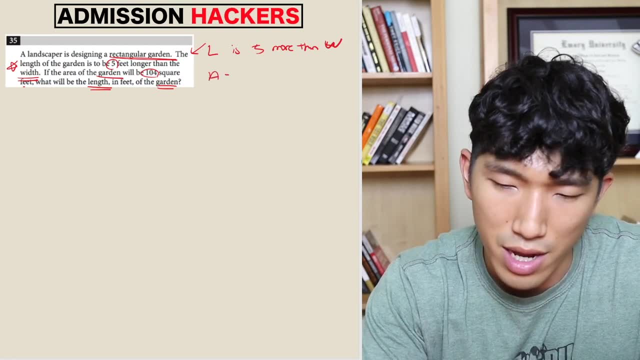 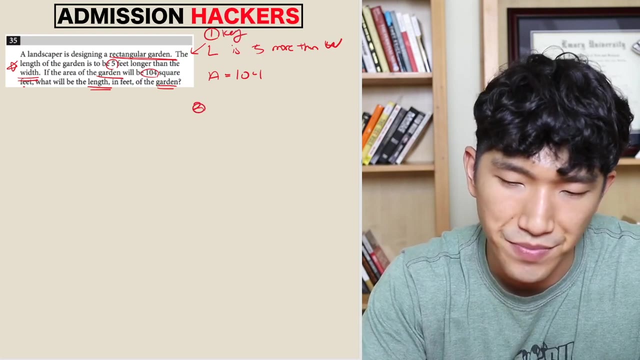 information that we have. what we know so far is that length is five more than w right and we know that area is going to be 104. okay, so that's going to be our key information and from this we're going to make two equations. okay, so length is five more than width. that looks like length is. 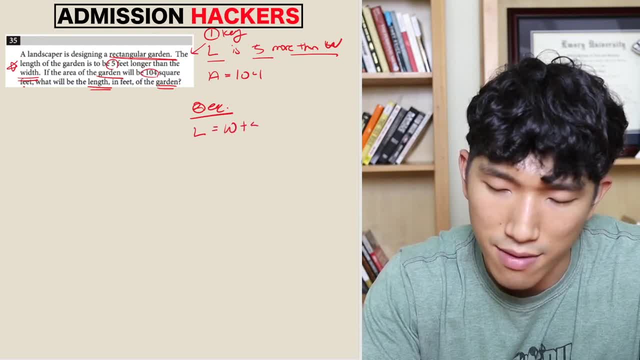 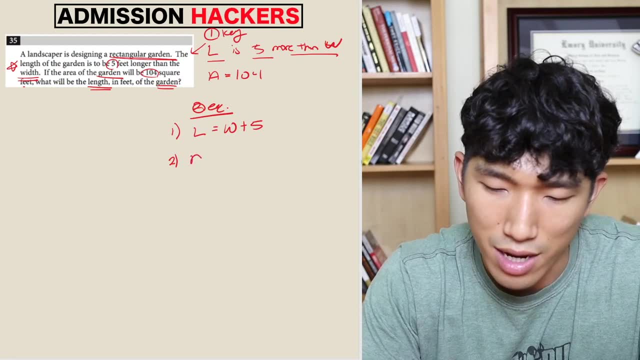 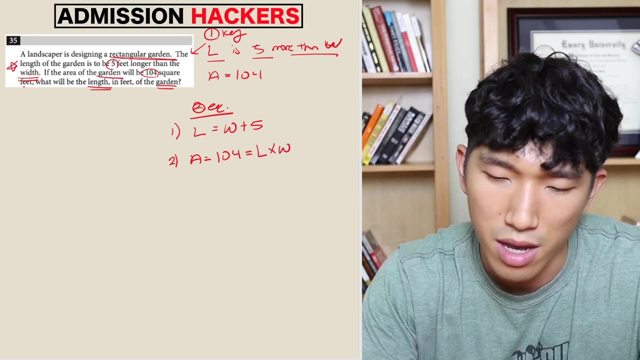 five more. so there's width and there's five more than width. okay, so that's going to be our first equation and second one equation. second equation is going to be our area. right area is going to be 104, and how do we get? area is going to be length times width. okay, so that's going to be our second. 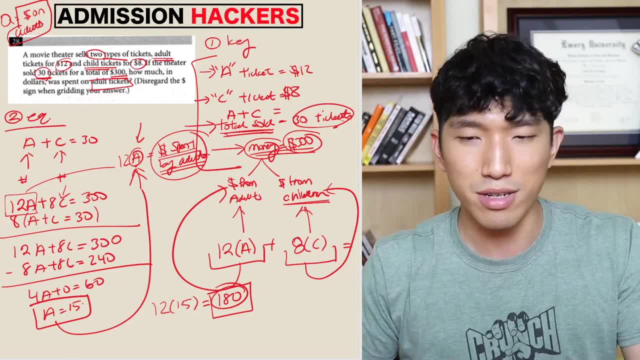 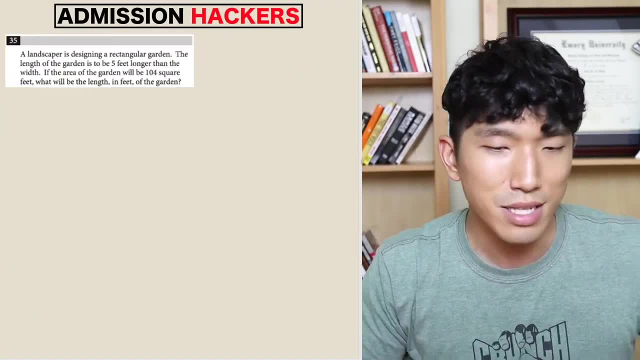 spent. total of 180.. Make sense. So the first thing you do is identify the key information And then with that you make two equations and you use systems to solve again. Let's go to the last one. A landscaper is designing a rectangular garden and the length of the garden is to be: 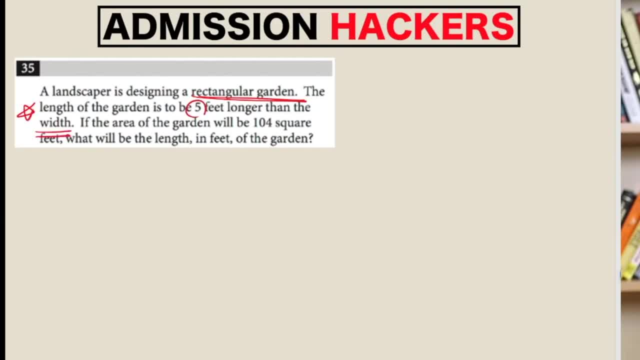 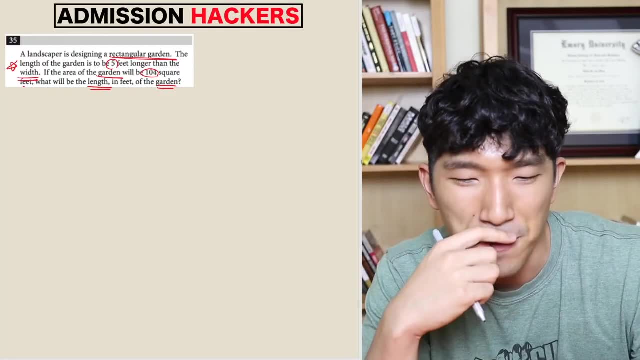 five feet longer than the width. Okay, That sounds pretty important. If the area of the garden will be 104 square feet, what will be the length and feet of the garden? Right? So let's think about this based on the information that we have. What we know so far is that length is five. 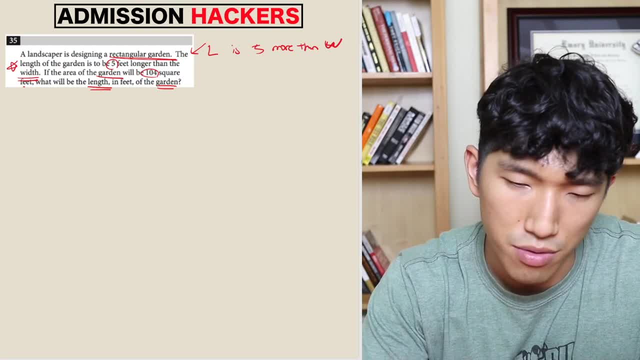 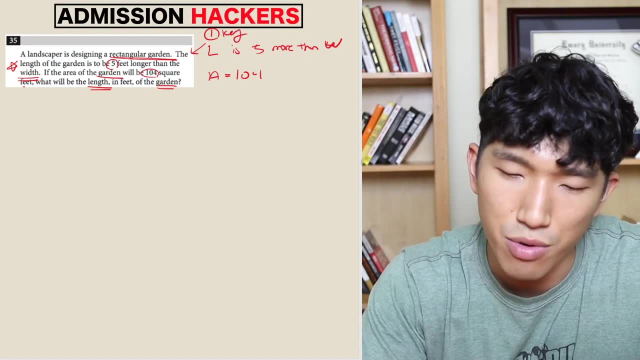 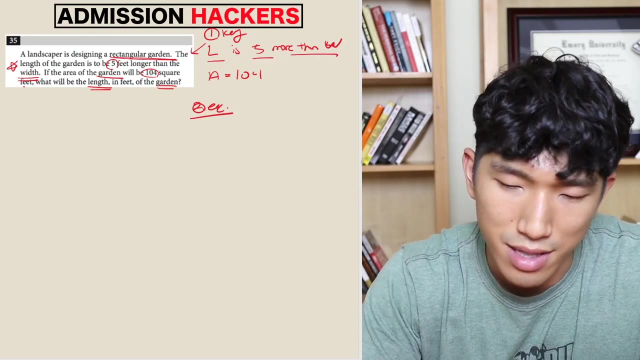 more than W, right, And we know that area is going to be 104.. Okay, So that's going to be our key information And from this we're going to make two equations. So length is five more than width. That looks like length is five more. So there's width and 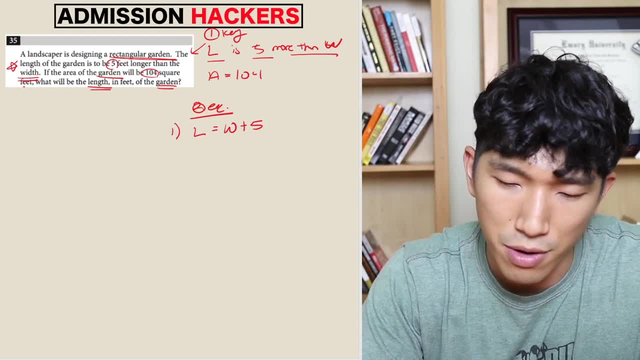 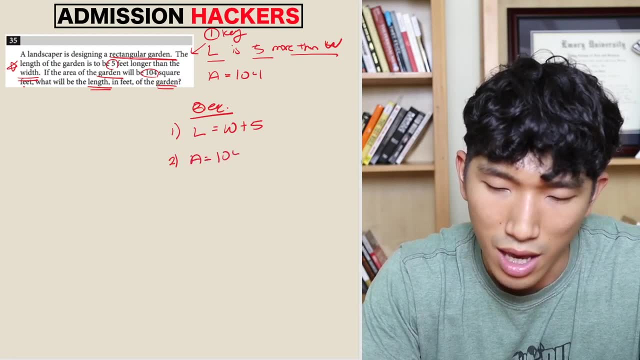 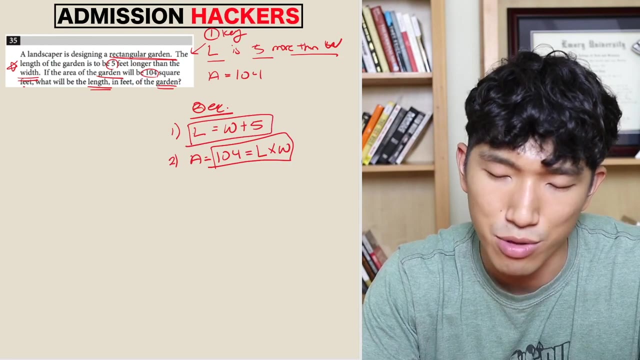 there's five more than width. So that's going to be our first equation And second one. the second equation is going to be our area. right Area is going to be 104.. And how do we get area? It's going to be length times width. Okay, So that's going to be our second equation And this one's. 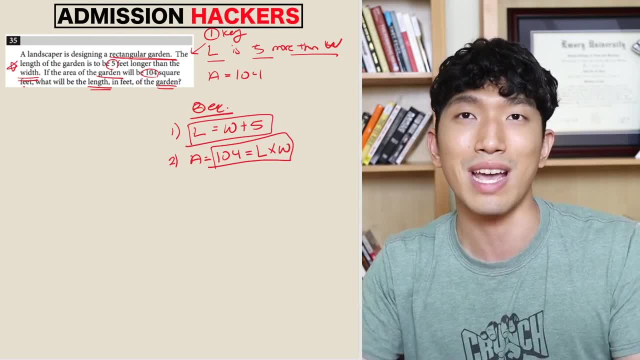 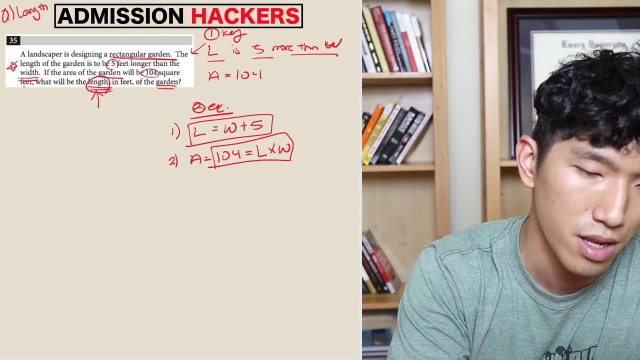 going to be our first equation and we're going to use this to find out what our answer is is and what are we looking for in this case, we are looking for the length, okay, so what we're looking for is what is length equal to? so what do we do? we try to get rid of w and find out exactly. 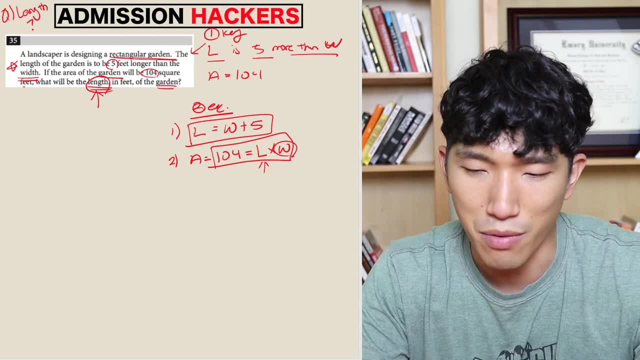 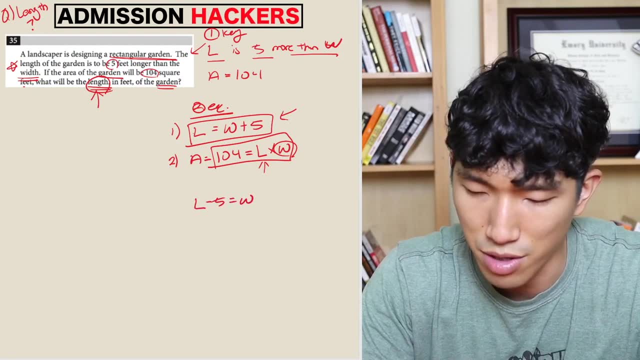 what l is. in this case we're going to use substitution. so how can we do that to eliminate w? what we're going to do is we're going to set the equation equal to w, so it's going to be: l minus 5 is equal to w, okay, and with this we're going to substitute it right in there, so 104. 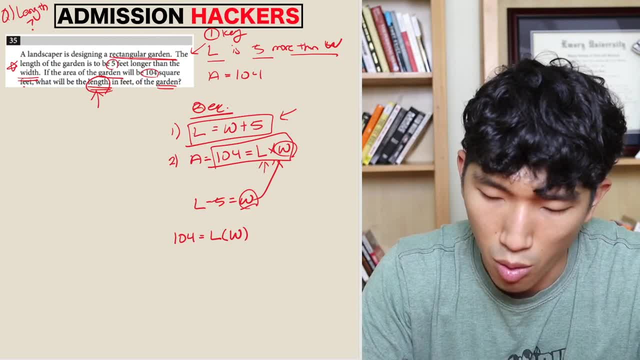 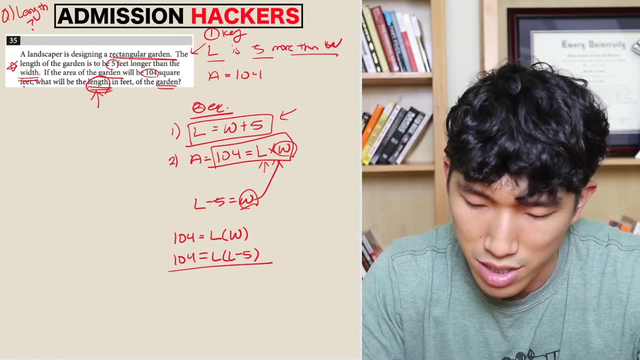 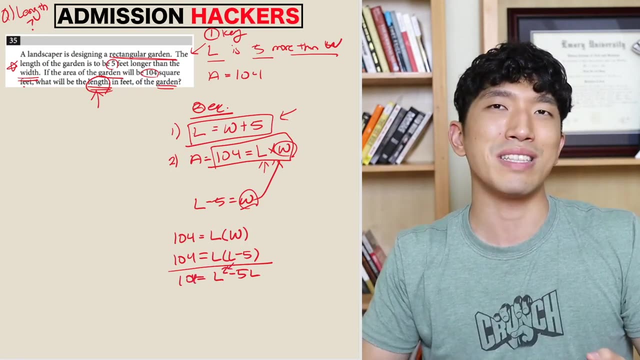 is equal to l times w, or same thing as l times l minus 5, right, and that's going to equal 104, and if you distribute this, you get l squared minus 5. l is equal to 104 and you see a square. so that probably means it has to do something with quadratics. and for quadratics, what do you do? you? 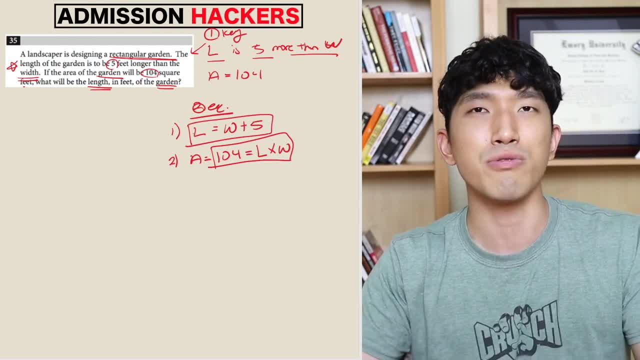 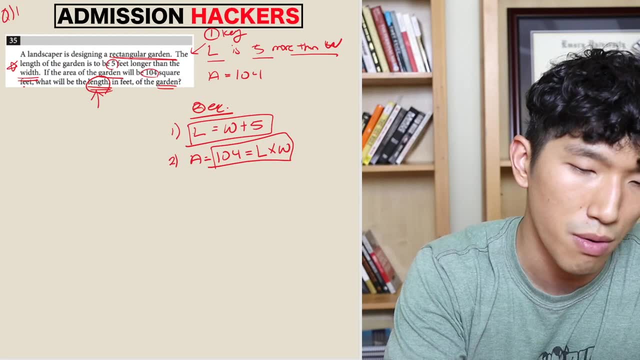 second equation- and this one's going to be our first equation, and we're going to use this to find out what our answer is. and what are we looking for in this case? we are looking for the length, okay, so what we're looking for is what is length equal to? 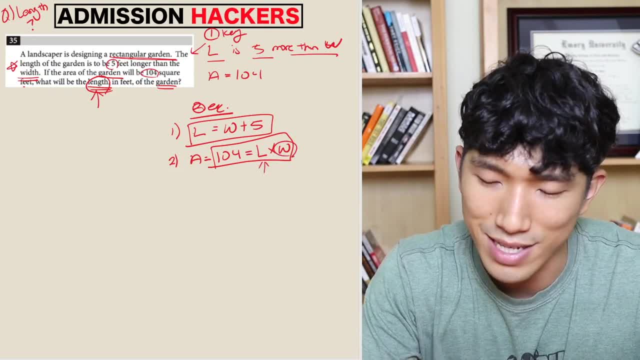 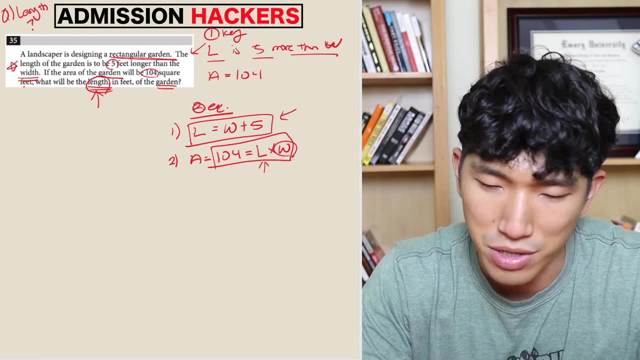 so what do we do? we try to get rid of w and find out exactly what l is. in this case, we're going to use substitution. so how can we do that to eliminate w? what we're going to do is we're going to set the equation equal to w, so it's going to be: l minus five is equal to w, okay, and with this we're. 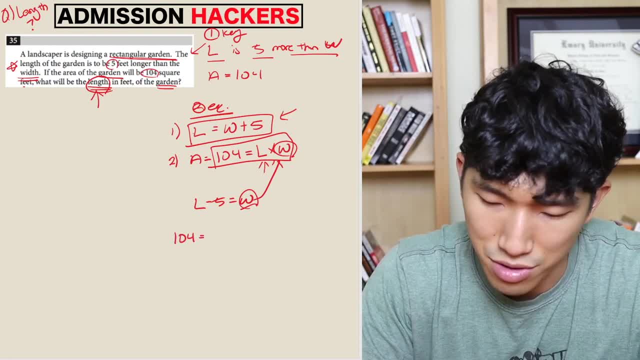 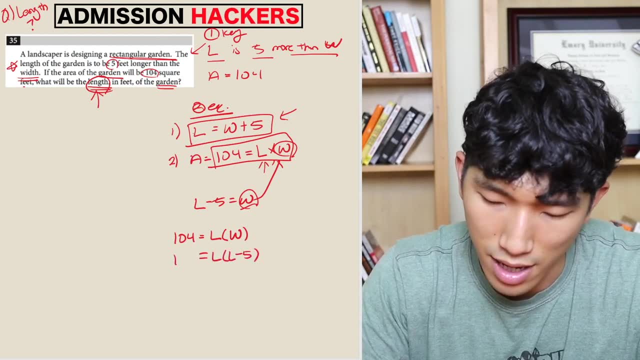 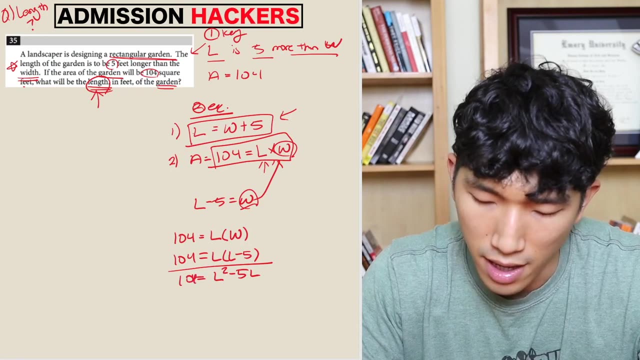 going to substitute it right in there. so 104 is equal to l times w, or same thing as l times l minus five. right, and that's going to equal 104. and if you distribute this, you get l squared minus five. l is equal to 104 and you see a square. so 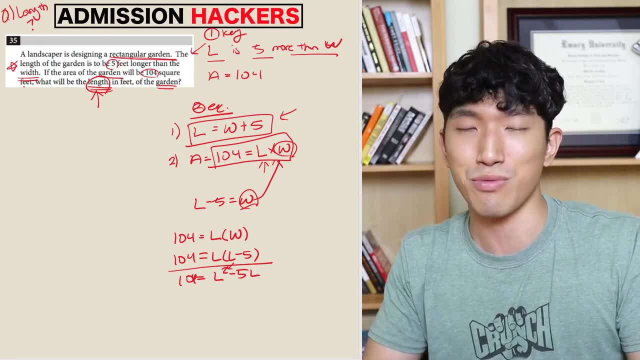 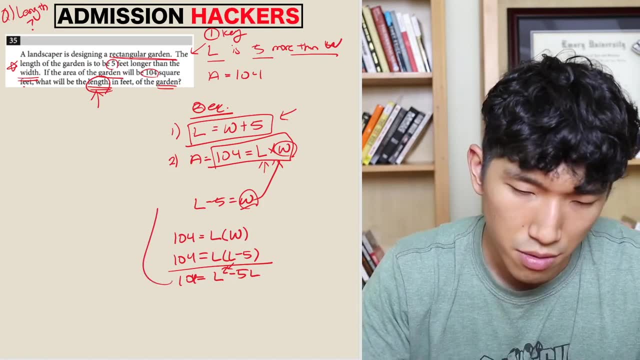 that probably means it has to do something with quadratics. and if, for quadratics, what do you do? you have to set it equal to zero to find out what the answer is. if that doesn't make sense, check out the quadratics video linked above. so let's just move this up here. and if we move the 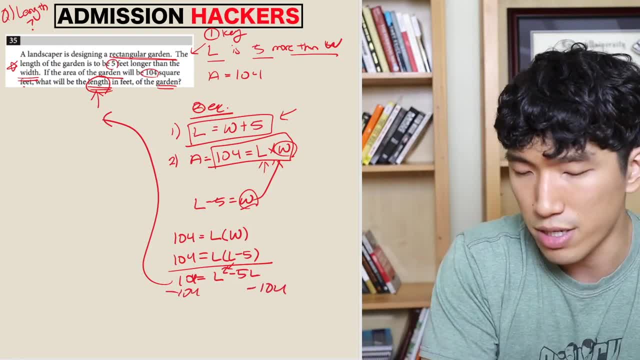 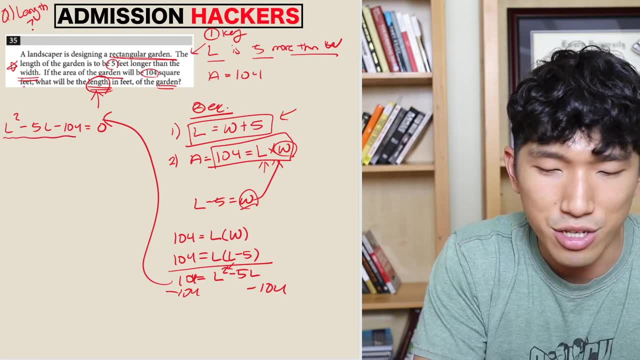 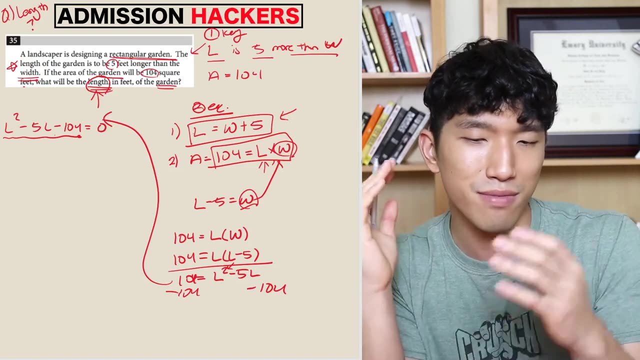 104 to the other side, then our equation is going to look like l squared minus five. l minus 104 is equal to zero, and all we have to do now is just factor this and you can find out exactly what your answer is. but 104 is a big number. it might be a little bit tough for us to factor it and what you. 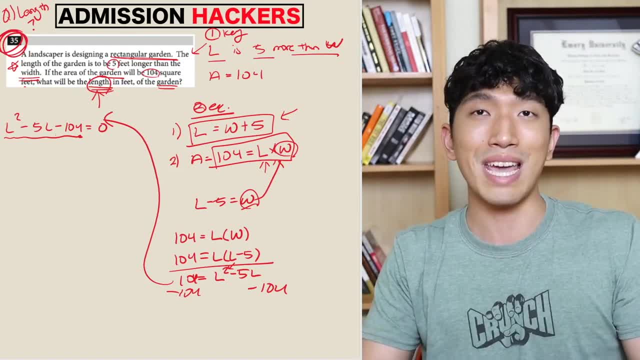 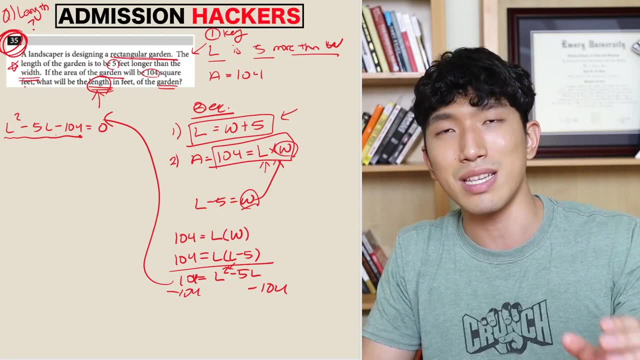 can see is that it's a 30, number 35, which means it's from a calculator section, because section three, no calculator section, only has up until 20 questions. so number 35, it means it's a calculator section, which means we can use our calculator. so let's use our calculator to factor. 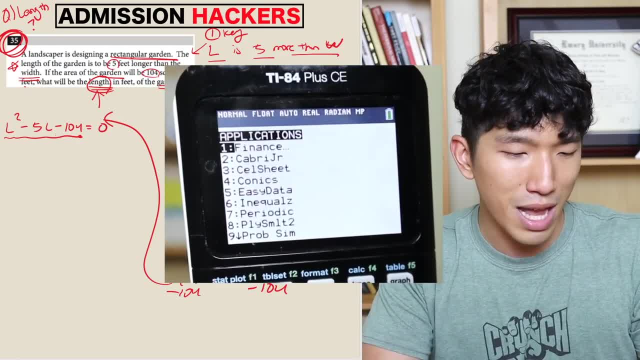 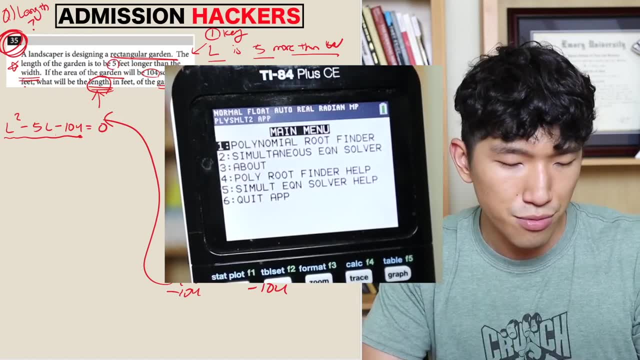 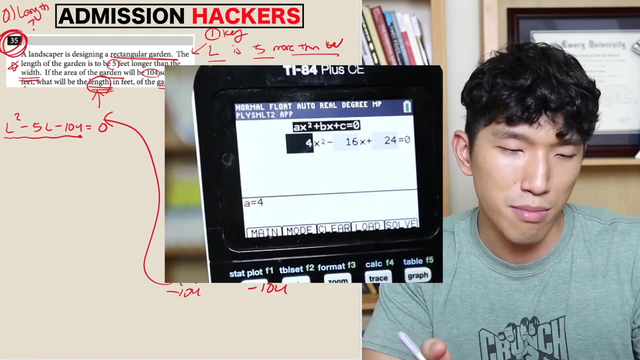 so how you do that is: you first go to apps and if you go down to number eight you're going to see a poly, smlt2. that stands for a polynomial simulator, and the first one says polynomial root finder. go into that and just make sure your screen looks like that and you hit next and you just plug in. 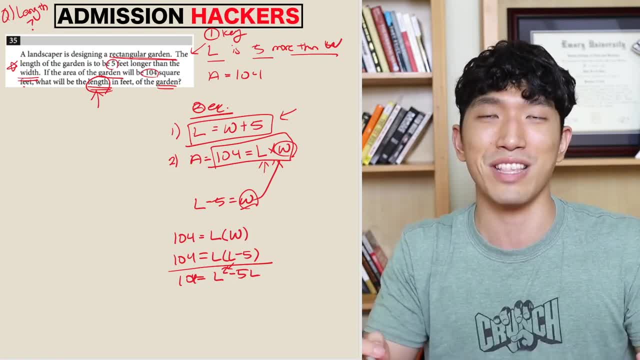 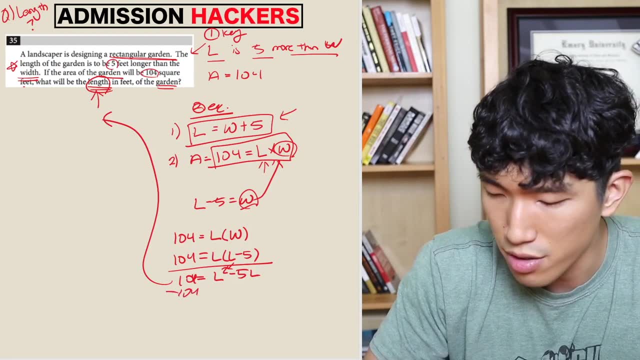 have to set it equal to zero to find out what the answer is. if that doesn't make sense, check out the quadratics video linked above. so let's just move this up here. and if we move more 104 to the other side, then our equation is going to look like L squared minus 5L minus 104. 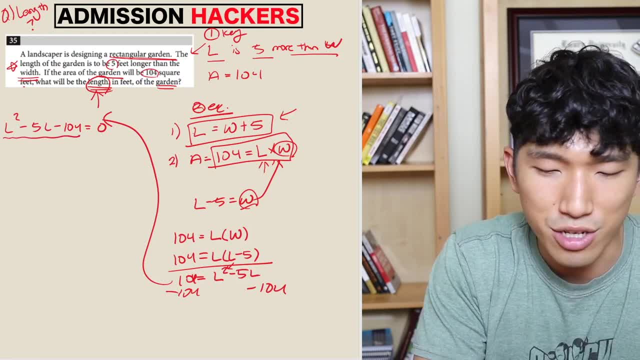 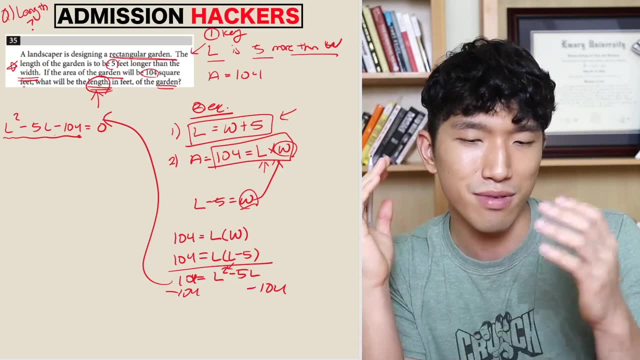 is equal to 0. And all we have to do now is just factor this and you can find out exactly what your answer is. But 104 is a big number. It might be a little bit tough for us to factor it, And what you can see is that it's a 30 number- 35,- which means it's from a calculator section, because 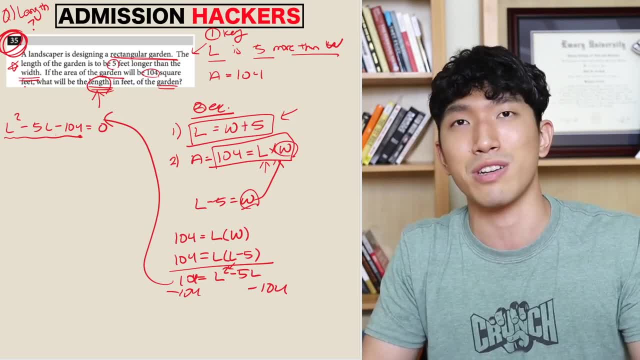 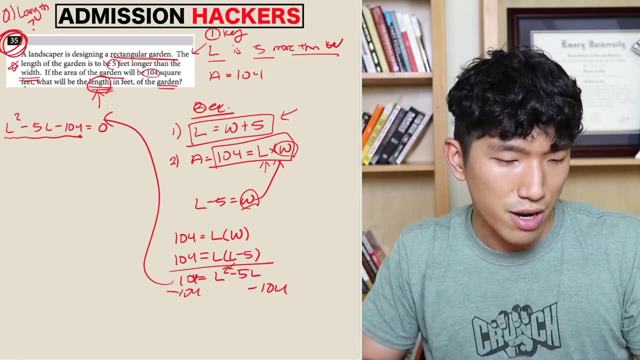 section 3, no calculator section only has up until 20 questions, So number 35, it means it's a calculator section, which means we can use our calculator. So let's use our calculator to factor. So how you do that is you first go to apps And if you go down to number eight you're going to see. 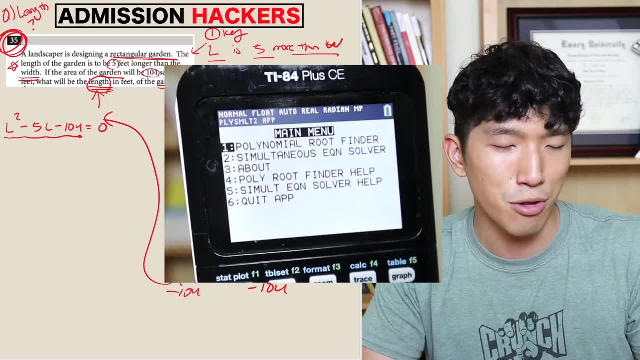 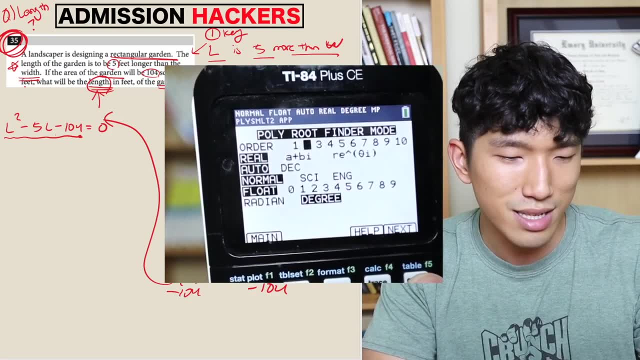 a polysmlt2.. That stands for a polynomial simulator And the first one says polynomial root finder. go into that and just make sure your screen looks like that And you hit next And you just plug in numbers based on what your equation is. Okay, so our L, or coefficient of L, 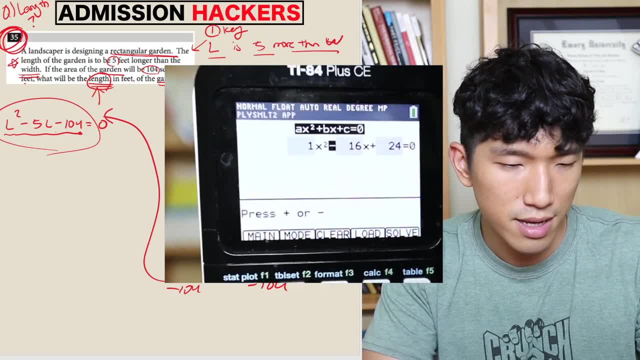 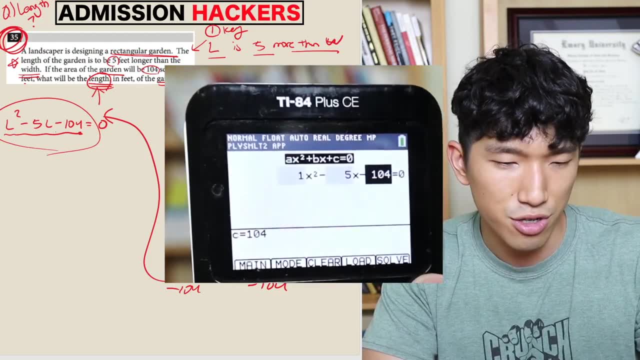 squared is going to be one, So we just put one And it's minus and minus five, minus 104.. And after you do that, you hit the graph button, which stands for solving, And if you solve it you find out that our L value can either equal: 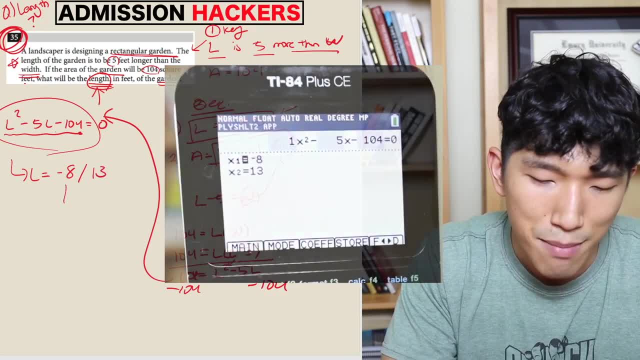 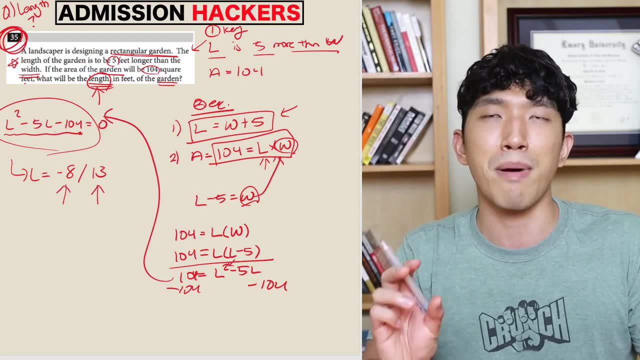 minus L, minus eight or 13.. Okay, that means our length can either be minus eight or 13. But can both of them be our answers? And that is no, it can't. Only a positive number can be an answer for a free response question. But more importantly, how can you have a length of minus? 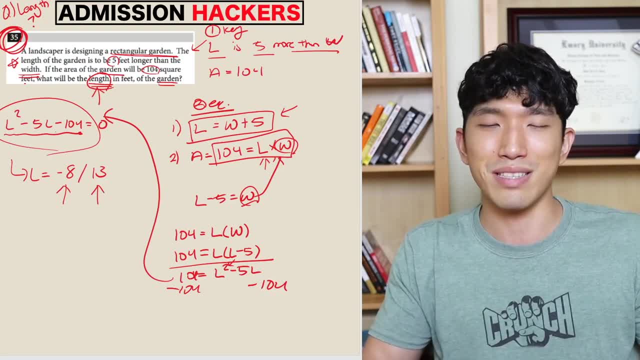 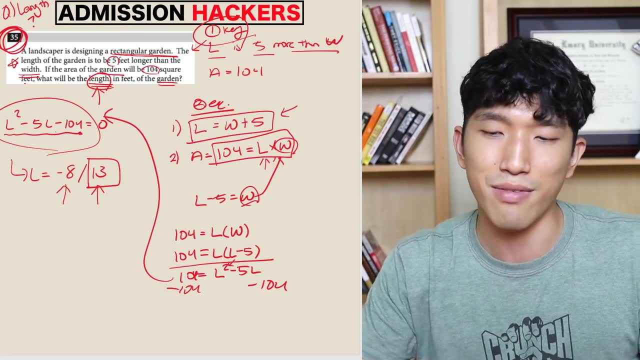 eight, like it's minus eight inches long. What does that even mean? Doesn't make sense. Okay, so our answer is going to be 13.. Does that make sense? So it's the same thing over and over again: First identify the key information and then solve. make the equations and solve for it using. 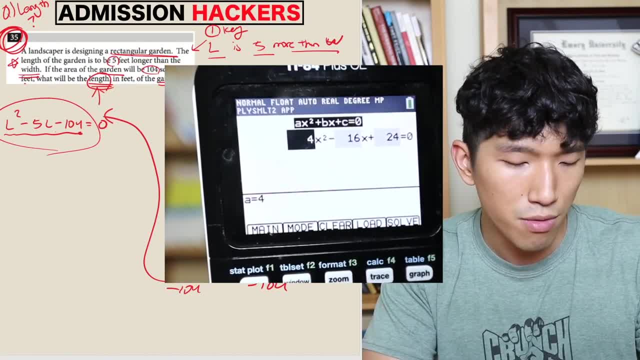 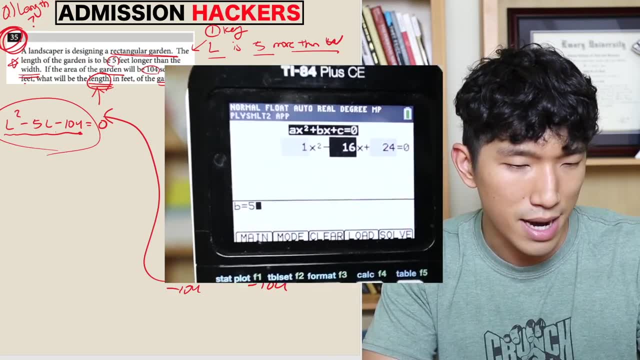 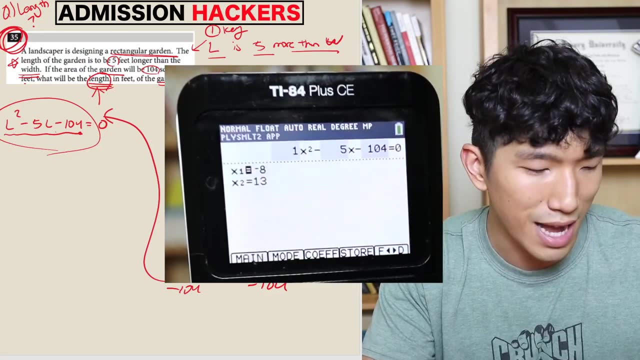 numbers based on what your equation is. okay, so our l, or coefficient of l squared, is going to be one, and it's minus and minus five, minus 104. and after you do that, you hit the graph button, which stands for solving, and if you solve it, you find out that our l value can either equal minus l, minus eight. 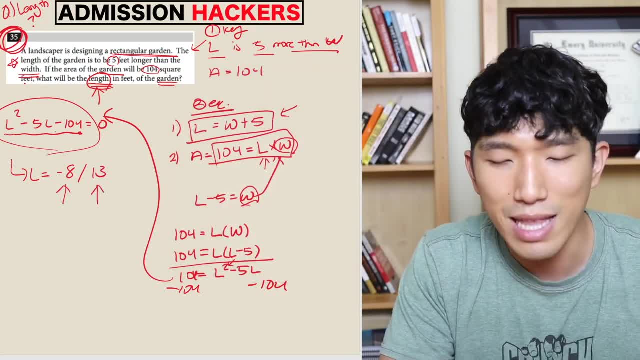 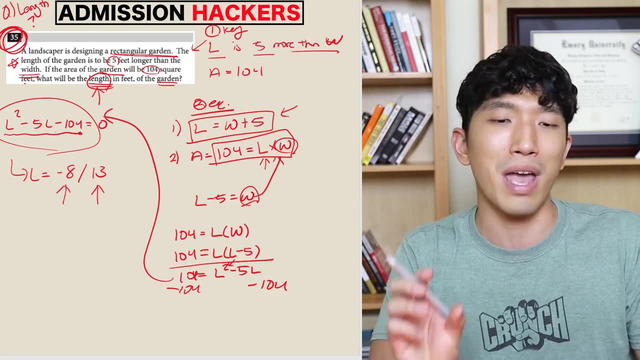 or 13. okay, that means our length can either be minus eight or 13, but can both of them be our answers? and that is no, it can't. only a positive number can be an answer for a free response question. but more importantly, how can you have a length of minus? 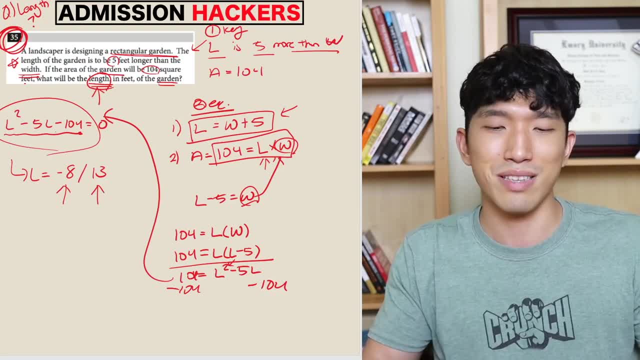 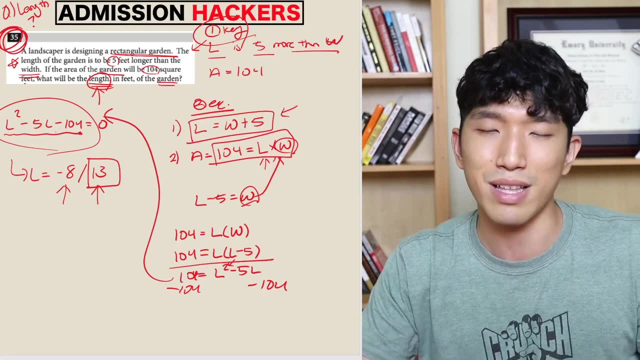 eight, like it's minus eight inches long. what does that even mean? doesn't make sense. okay, so our answer is going to be 13. does that make sense? so it's the same thing over and over again: first identify the key information and then solve. make the equations and solve for it using a systems. 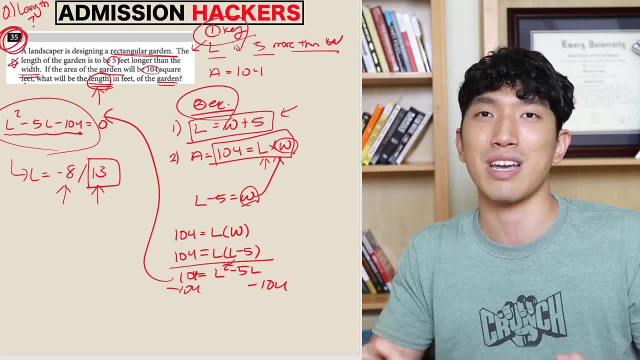 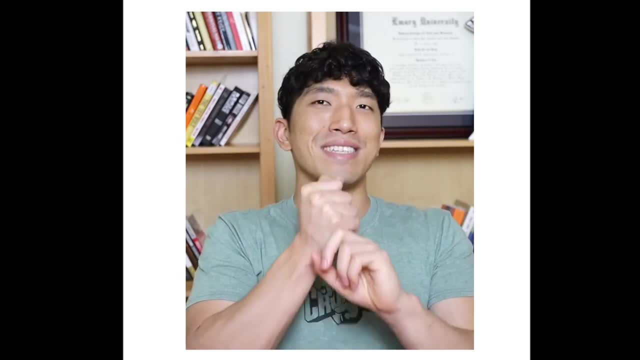 of equations. if you don't know what systems of equation is, make sure you check out the lecture- it's up there somewhere, i think, and that's exactly how you solve these square problems. what you want to do is first identify exactly what the key informations are and, based on those key informations, 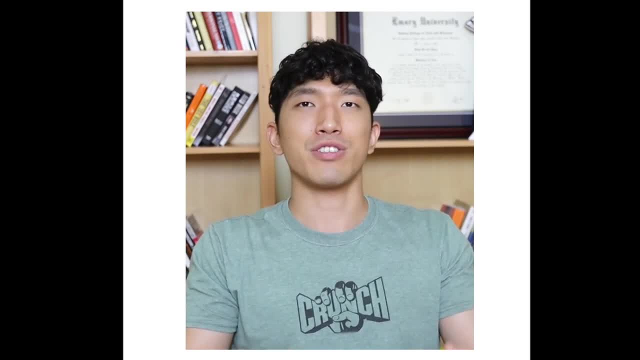 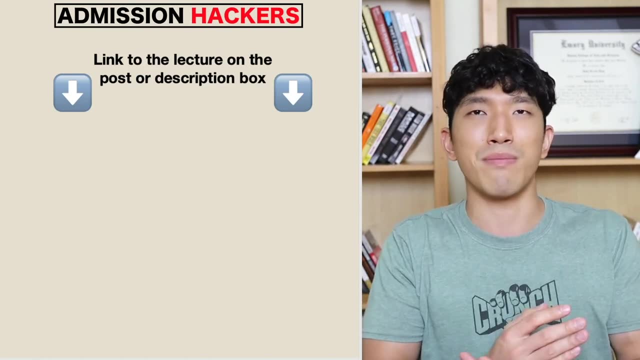 you have to create a equations from that and just use those equations and you should be able to find out exactly what your answer is. honestly, i could have gone more in detail into each steps in this problem, but that would have made the video 40 minutes long. however, if you want to really master these word problems, 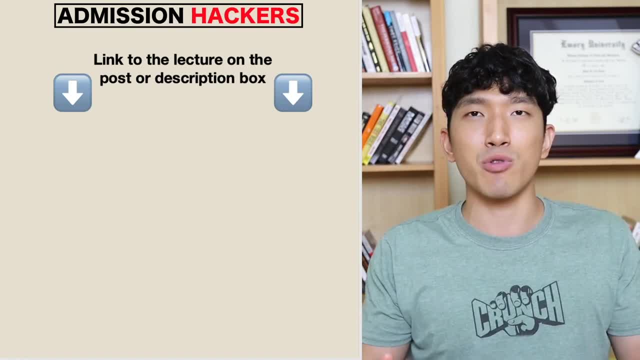 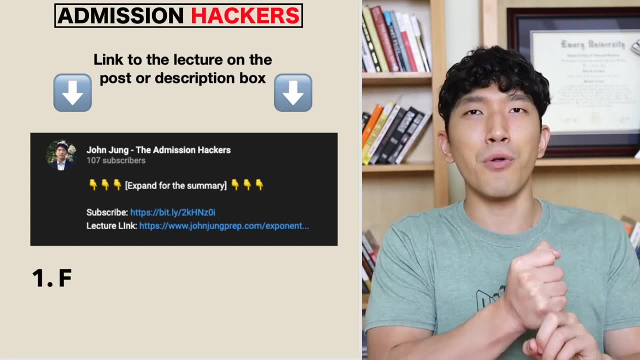 and go deep down into the explanations by step by step. then there's going to be a link in the description box down below and it's going to take you to a private lecture. and in the lecture you're going to get three things. first you're going to get a full-length lecture on word problems. how? 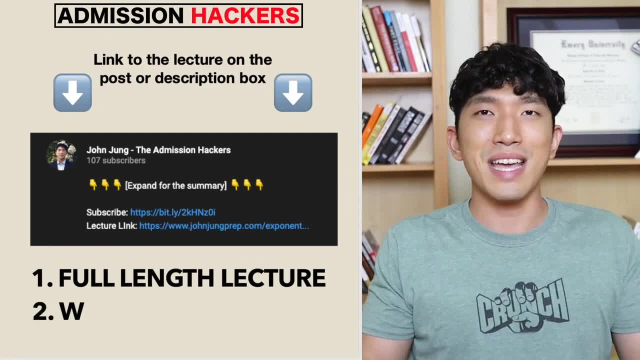 to approach them, how to solve them step by step, explain and second, there's also going to be a worksheet that you're going to be able to use to solve these problems and you're going to be able to get a full-length lecture on word problems that goes along with the lecture, which you can print out. 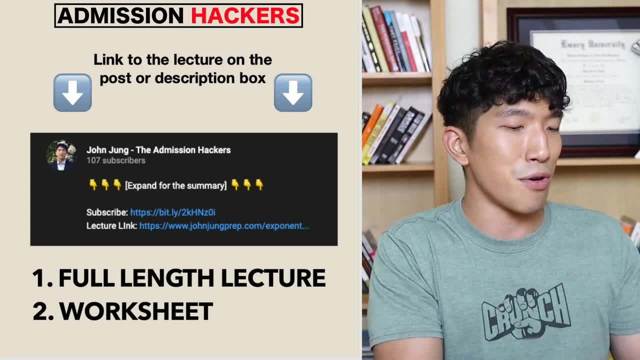 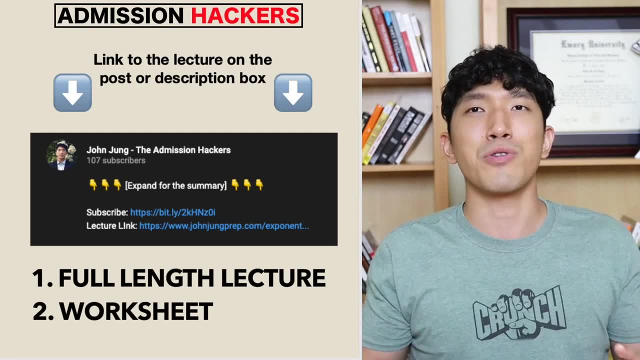 and follow along the video with it, and also it's going to exactly point out what you need to know, those little tips and tricks to solve these word problems, so they are going to be really helpful. and, last but not least, there's also going to be a set of practice questions at the end of 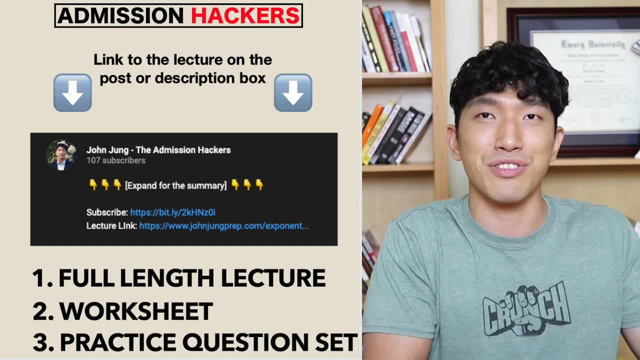 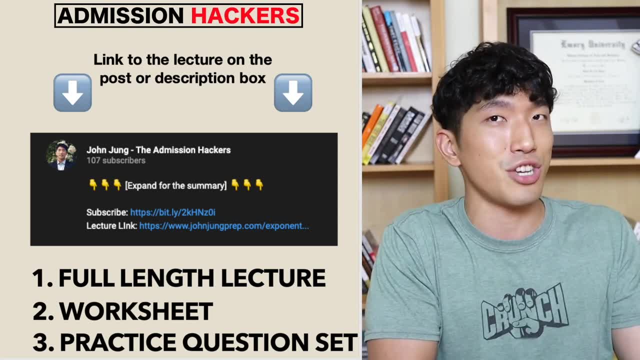 the lecture where you can try out these word problems to see if you really understood how to solve these word problems. and they are just a collection of actual sat word problems. so if you can solve those questions, i think you're in a pretty good shape. anyways, guys, that's going. 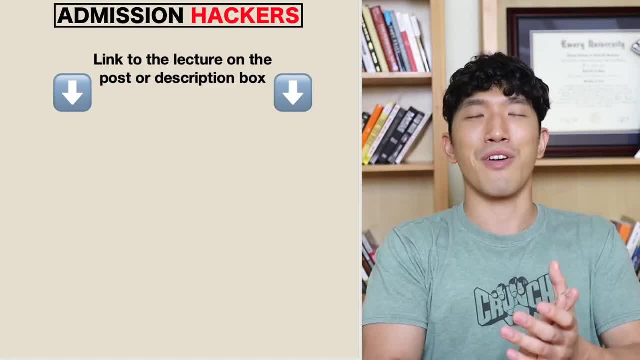 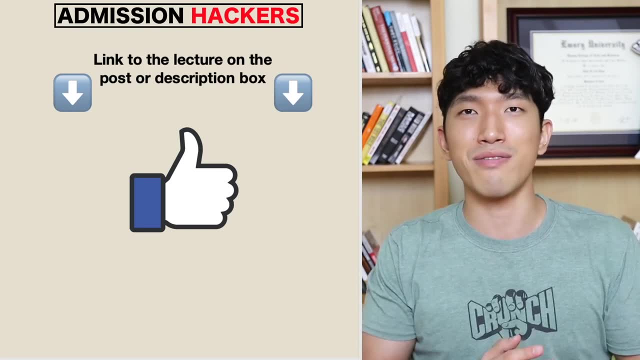 to be it for today's video. if you guys made it until the end, very proud of you. not many people actually made it till the end. if you guys like this video or found this video helpful at all, make sure you guys smash the like button and if you love this kind of. 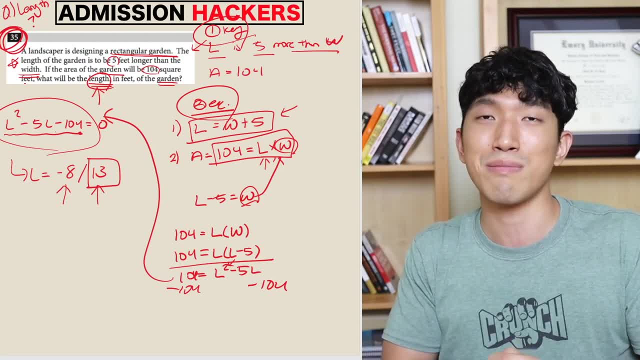 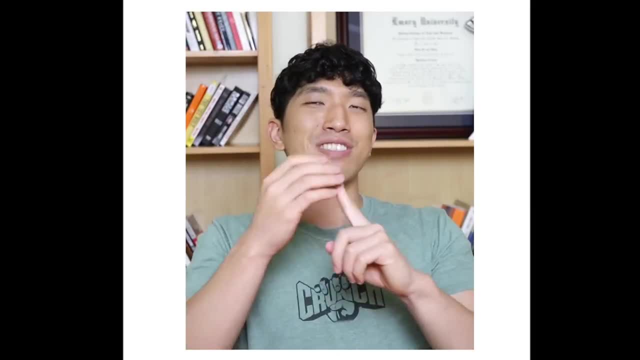 a systems of equations. If you don't know what systems of equation is, make sure you check out. the lecture is up there somewhere, I think, And that's exactly how you solve these square problems. What you want to do is first identify exactly what the key informations are And based 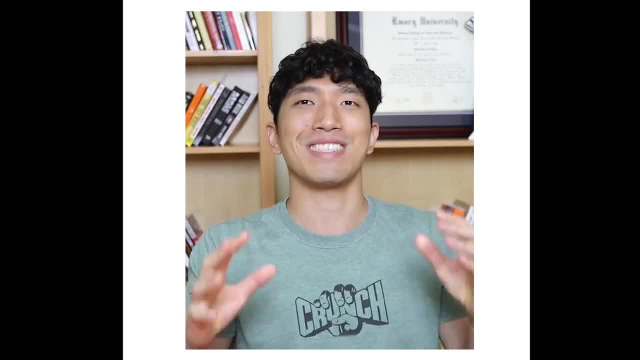 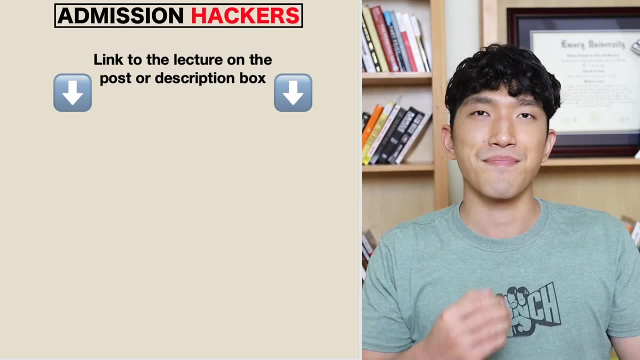 on that, you should be able to find out exactly what your answer is. Honestly, I could have gone more in detail into each step in this problem, but that would have made the video 40 minutes long. However, if you want to really master these word problems and go deep down into the explanations, 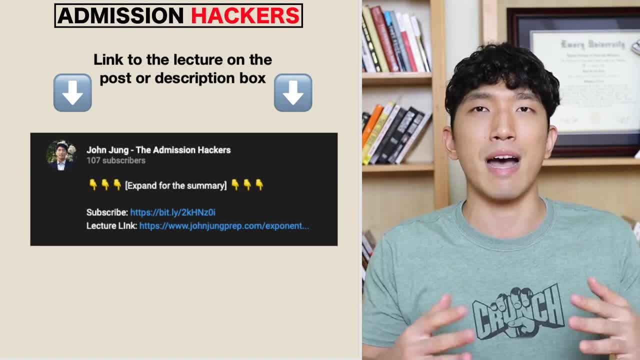 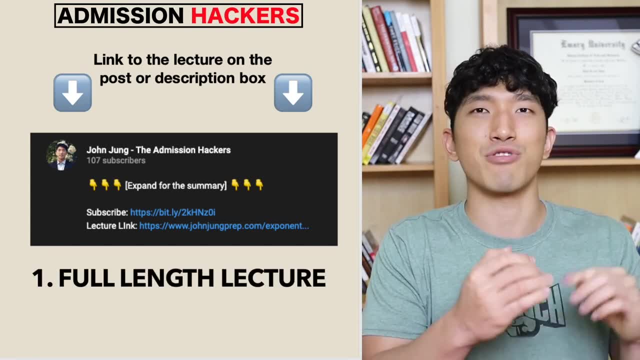 by step by step. then there's going to be a link in the description box down below And it's going to take you to a private lecture. And in the lecture you're going to get three things. First, you're going to get a full length lecture on word problems, how to approach them, how to solve them. 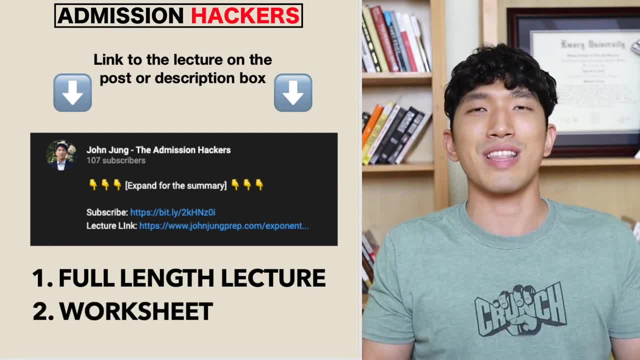 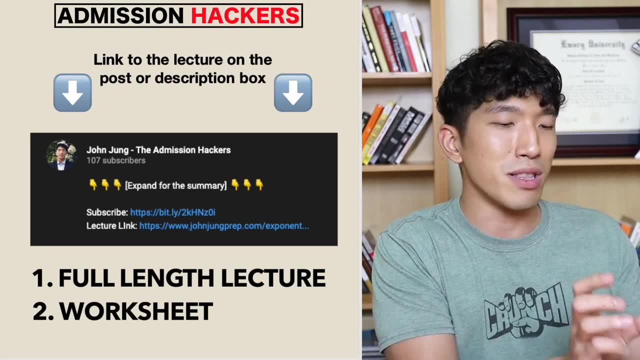 step by step explained. And second, there's also going to be a worksheet that goes along with the lecture, which you can print out and follow along the video with it, And also it's going to exactly point out what you need to know, those little tips and tricks to. 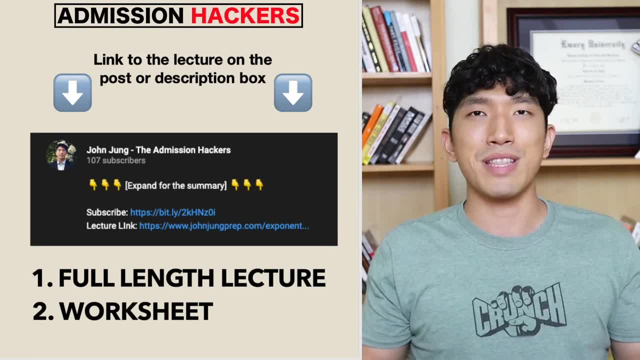 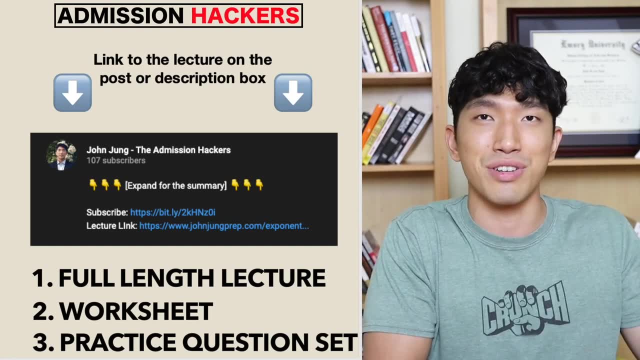 solve these word problems. So they're going to be really helpful. And, last but not least, there's also going to be a set of practice questions at the end of the lecture where you can try out these word problems to see if you really understood how to solve these word problems. And they are just a. 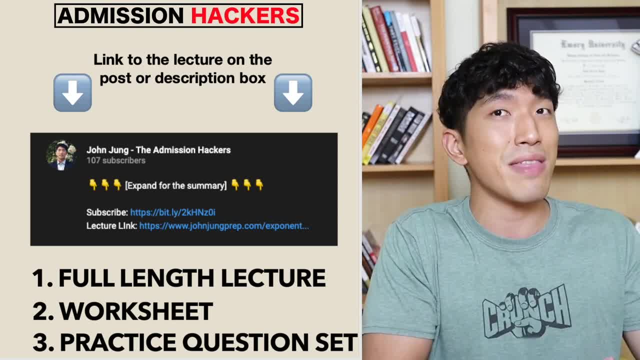 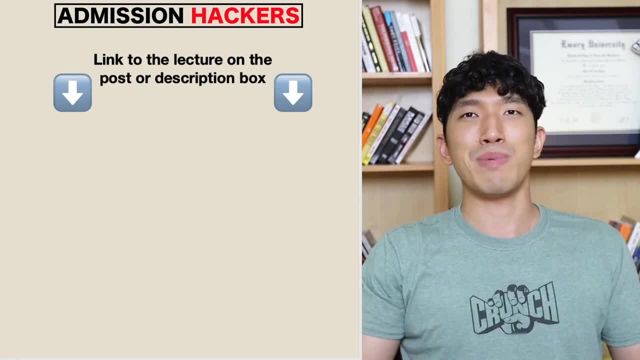 collection of actual SAT word problems. So if you can solve those questions, I think you're in a pretty good shape. Anyways, guys, that's going to be it for today's video. If you guys made it until the end, Very proud of you. Not many people actually made it till the end. If you guys liked this video or 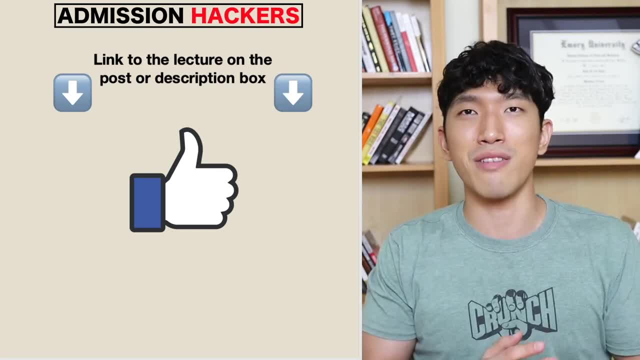 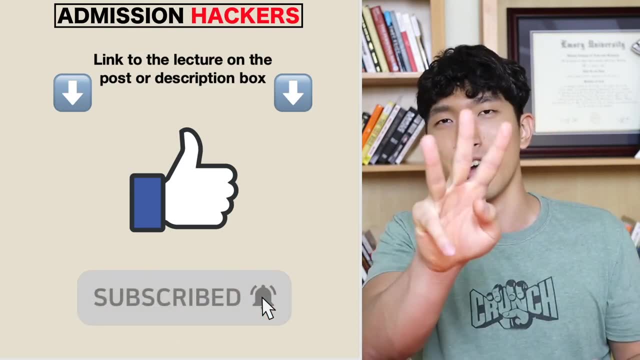 found this video helpful at all. make sure you guys smash the like button And if you love this kind of content and would love to see more, I would highly suggest you subscribe to the channel, because every Monday, Wednesday, Friday at 3.30pm I release these videos summarizing exactly what 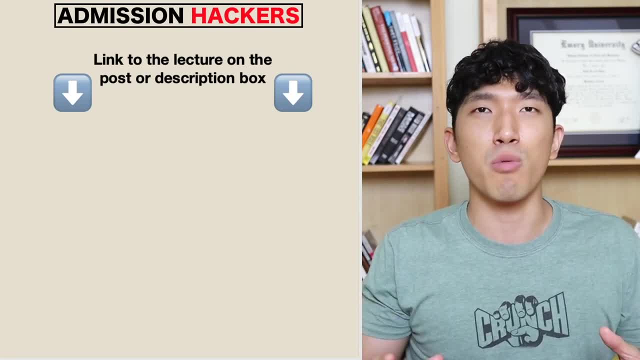 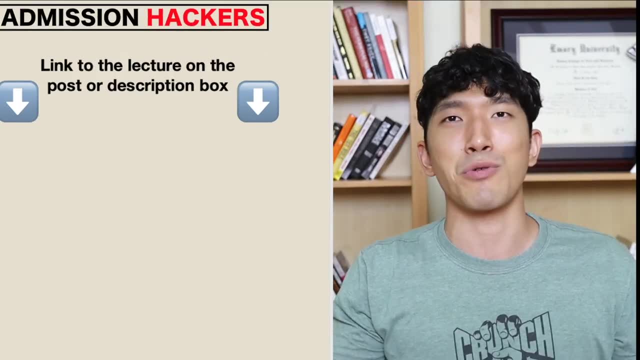 you need to know for the SAT section. Watching these videos alone will save you so much time- all the time that you would spend going over these test spread books trying to understand exactly what you need to know for the SAT. If you guys have any questions or comments, 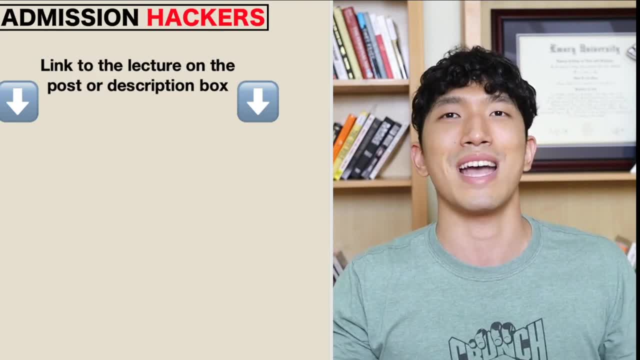 leave it in the description box down below, And if there is something you want to see next, let me know in the comment box, because, as always, this channel is based on what you guys want to see and not what I want to talk about. Thank you so much for watching. I'll see you guys in the next video. Bye. 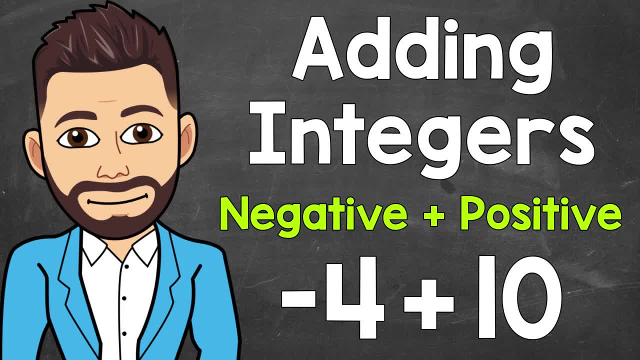 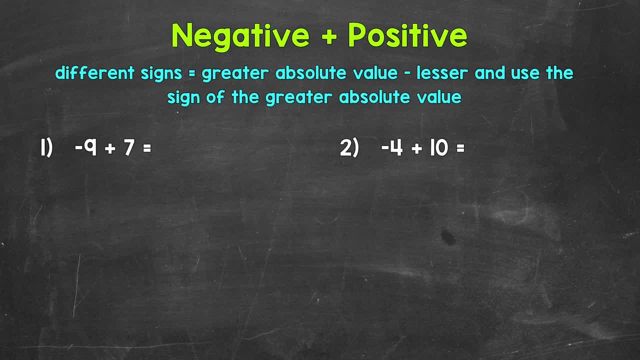 Welcome to Math with Mr J. In this video, I'm going to cover how to add a negative integer and a positive integer, So a negative plus a positive. Now, when it comes to adding integers, there are different ways to think through these. We will go through two ways for each of our